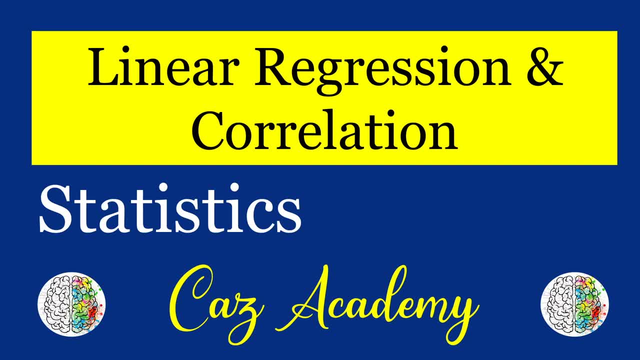 Welcome to today's statistics tutorial. Today we will be looking at linear regression and correlation. See the links below for the calculators and resources used in this tutorial, as well as additional supports and resources to help you with your statistics course Module 12, which is on linear regression. 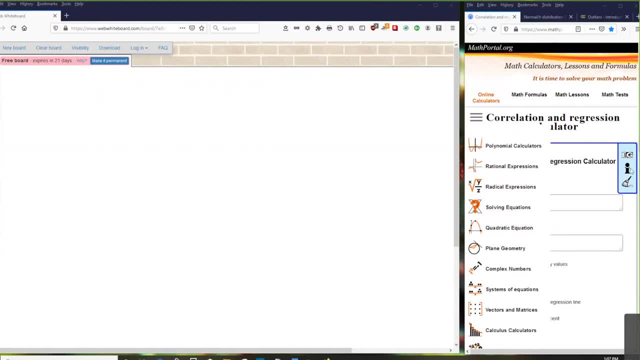 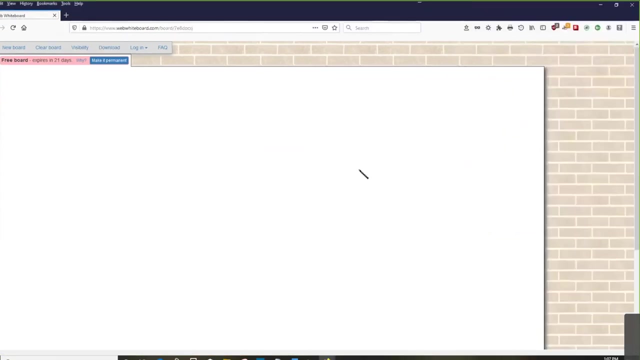 and correlation. So linear regression for two variables is based on a linear equation with one independent, which would be your X values, and your Y values, which would be your dependent variable, and your A and B are constant. So for statistics the formula is: Y equals A plus BX. So this is for statistics and you'll. 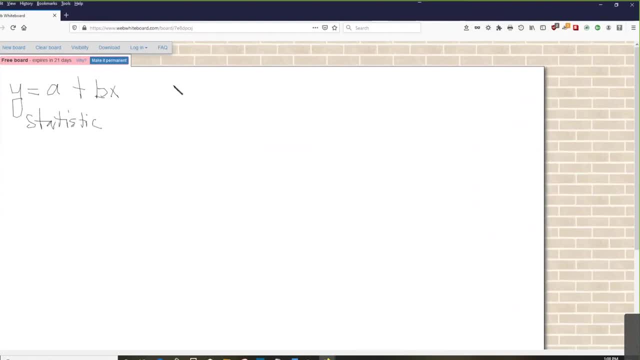 notice it looks very much like the Y equals M, X plus B formula that we use in algebra, which is the equations for a line, and these two are exactly the same. they're just written differently and that helps to identify. are you talking about something with statistics or are you talking about something for algebra? 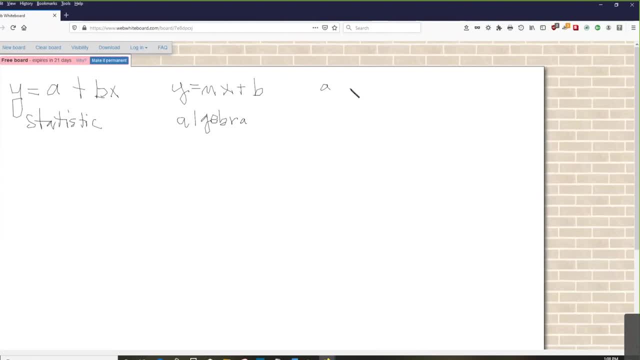 So your A from the statistic equation and your B from your algebra equation is your Y intercept, Or where you're, which is the value when X equals zero and it's where it crosses the line, And I did not give you the whiteboard link yet, so let me do that. 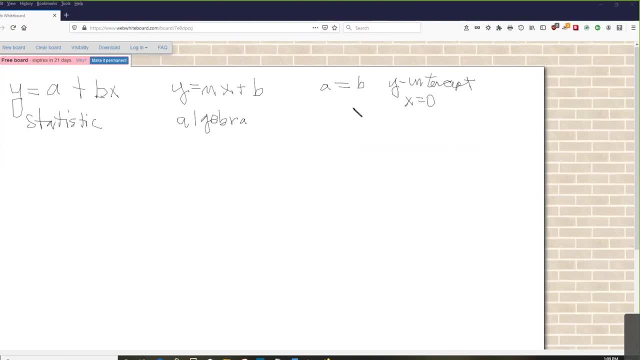 And then your, Your B of X on the statistic formula is the exact same thing as your MX on your algebra formula, and your B is going to equal your M, which equals your slope, Which just determines the steepness of the line. Okay, 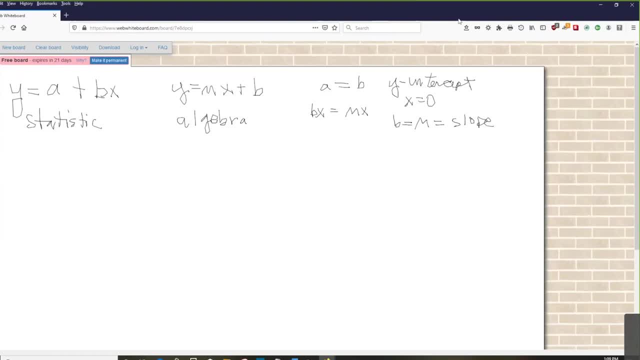 When you You have your data. so when you have your data, you're going to have your X and your Y. So it's just like what we've seen before with algebra, And then you're going to have scatter points and these are all going to have an X and a Y. 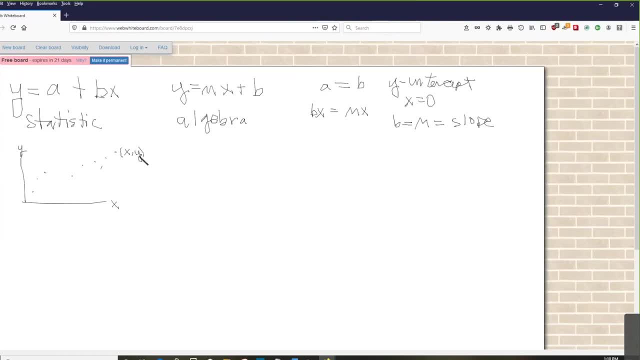 For each of these points it's going to have an X and a Y value, where X is going to be your independent. so that's what you choose independently, And then Y is considered dependent, because you plug in for whatever value of X you have. 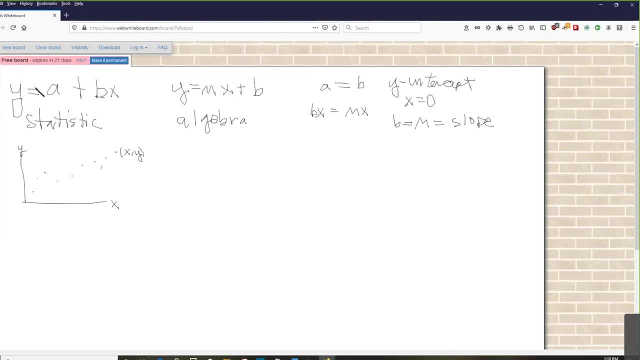 you're going to plug it into the equation to solve for Y. Then, with your data, you're going to plot your data on what is called a scatter plot, which we've seen before, and that just says you're going to put the point. 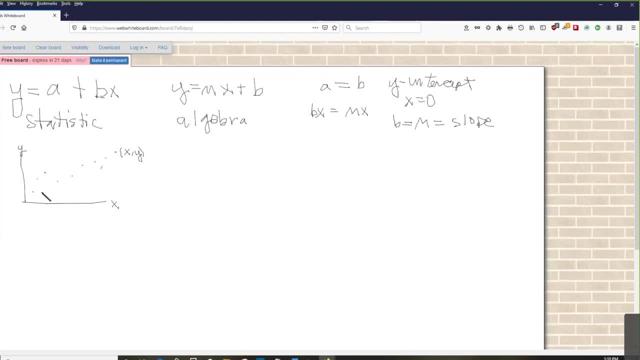 on a graph and see what it looks like. So if I have something That looks like this, this is going to be something that looks pretty close to a straight line, So that would be considered a strong positive linear pattern If I had one that looks similar. and then there was a point out here. 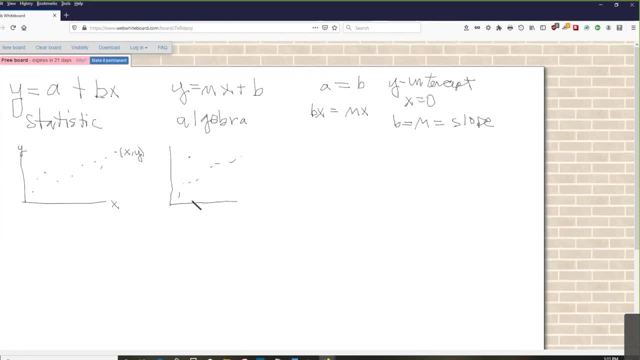 that would be a strong positive linear pattern with one deviation, because there's one that's a little away from what looks like a straight line. If I had, where they're all kind of spaced out big, but still kind of forming a line, this would be considered a weak correlation. 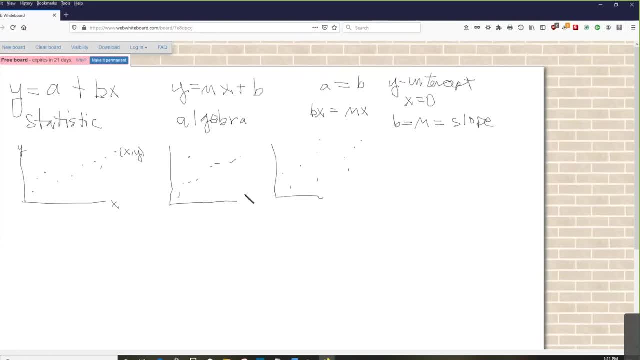 And so this would be because it's going to the right. any time you're going to the right, it's going to be considered positive. If I'm going the other direction, it's like something like this: this right here would be. 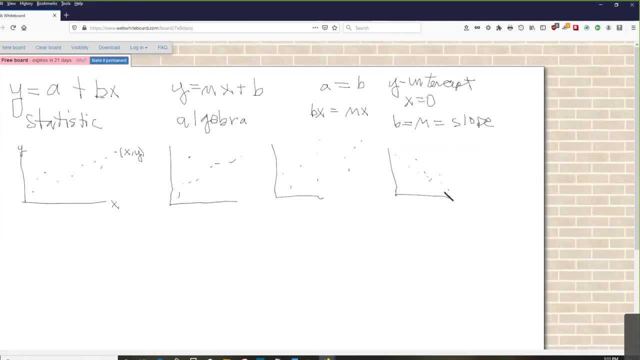 considered a strong negative linear pattern. Okay, So if it's going to go to the left, it's going to be considered negative. If it's going to the right, it's going to be considered positive. If I have one that's kind of staying on the bottom and then slowly comes up, 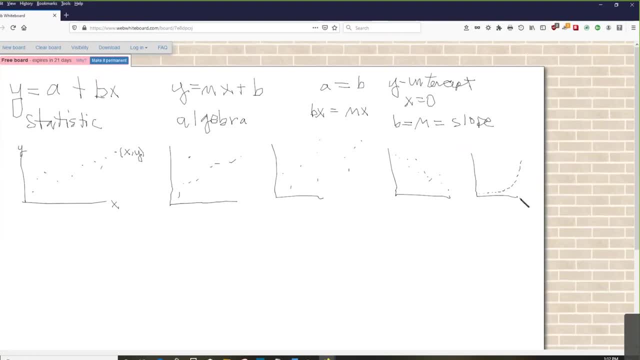 this is going to be an exponential growth pattern And that is not one that's going to fit this line, because it's a curve And if we have one where our data points are just going to be, they're just kind of all over the place, that would be considered to have no pattern. 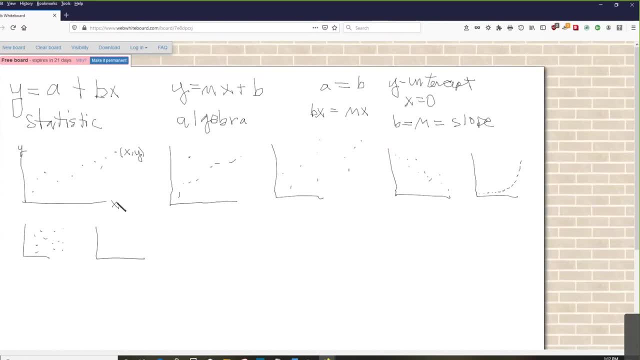 On our line. if we have. so, if I have a line going to the right, that is considered positive correlation And that means that the signs of my slope are going to be the same. They're either both going to be the same or they're going to be the same. 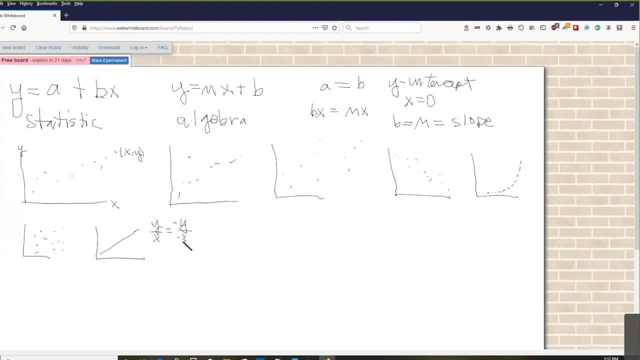 They're either going to be positive or they're both going to be negative, And that's going to be considered a positive correlation. If it goes the opposite direction, that's considered a negative correlation, And that just means that signs of my y and my x are going to be opposite. 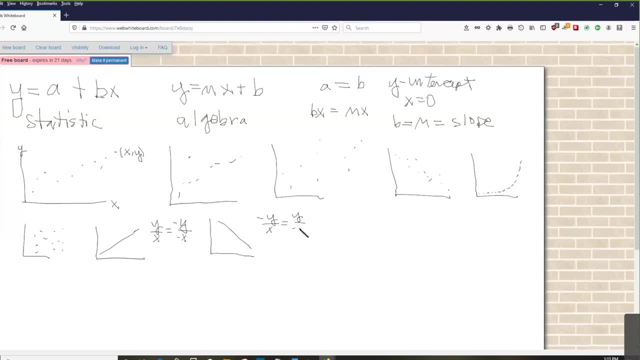 when I'm looking at my slope, So this is going to have a negative slope, which means it's going to be the same, So it's going to go to the left. And when I'm doing my solving for my y or my x's, they're going to be opposite. 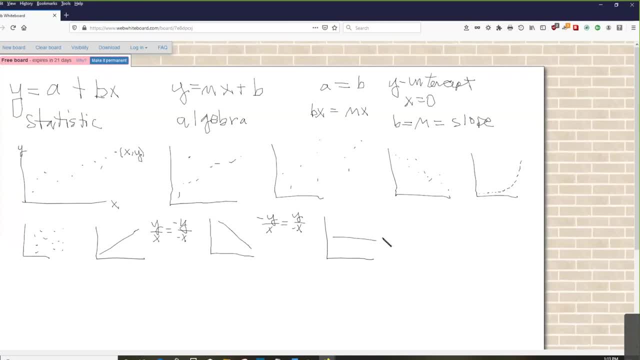 If it's a horizontal line, that's going to be considered a zero correlation or no correlation. And when we're solving these linear regressions, if the line has a curve to it, like we saw with this exponential growth, then it might also show up as having no correlation or zero correlation. 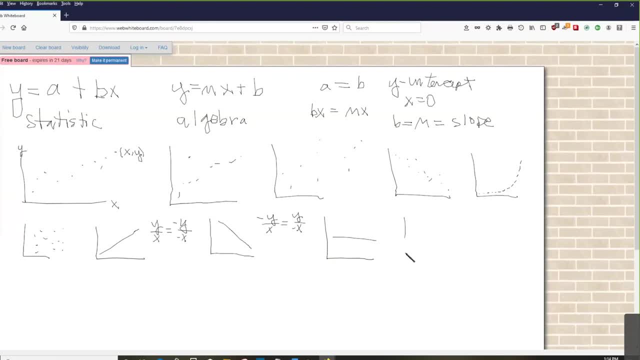 because it doesn't fit into a straight line. If I have a vertical line, that's considered undefined And that's because when we're doing the straight line, So anyway, so that is considered undefined, So you won't see that showing up at all. 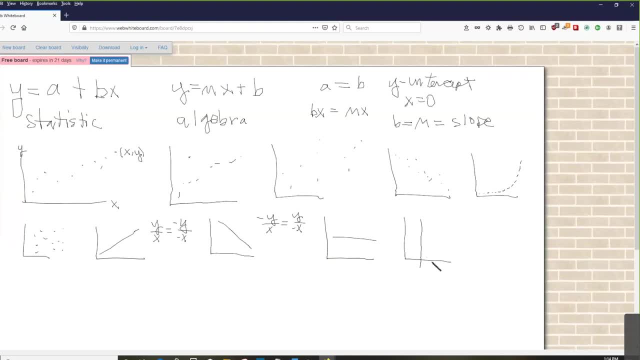 Now, if data has a linear relationship, we can use linear regression to draw a line that represents our relationship, given that one variable explains the other. Or, for a given x, we can use the regression line to predict y. So that's why we would want to use this- is that we can get two sets of values. 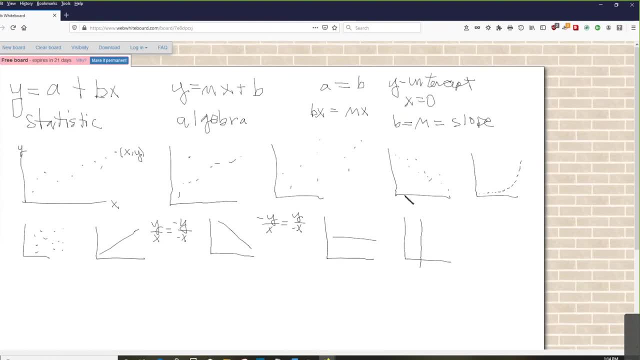 And let's see, Let's see, And let one be dependent on the other. If it looks like the data is going to have close to a linear or a straight line, then we can use it to predict possible outcomes, possible values. So if we have a set of data points that appear to fit a straight line, 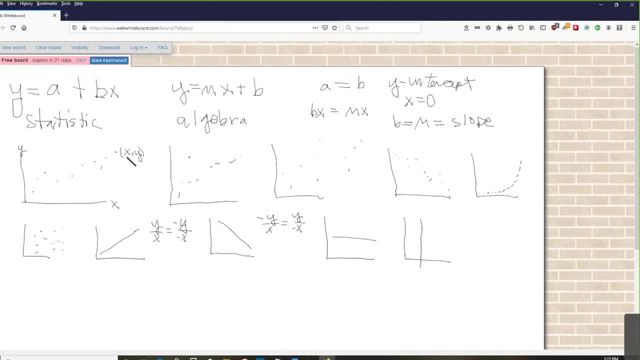 then this is called a line of best fit or least squares line. So if I have all of this data here and this kind of looks like it's going to be a straight line, so I can draw a straight line to represent all of these data points. 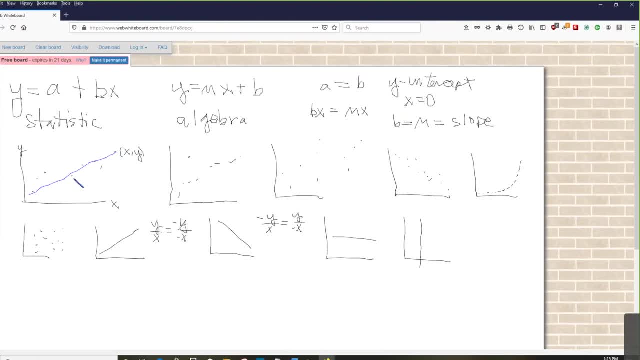 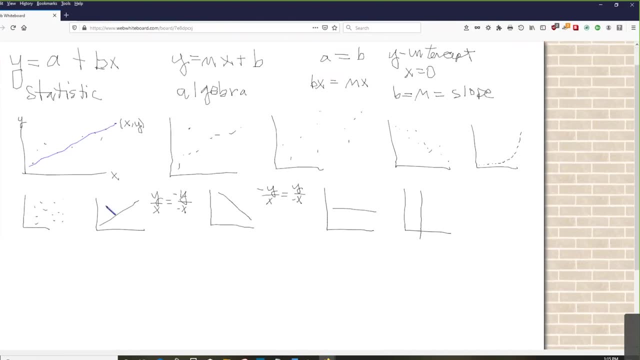 even though I've got some that are a little above, some that is below, And this is called the line of best fit or the least squares line, And we get this. So the way that we get this, and the Khan Academy has a really good video explaining these values- 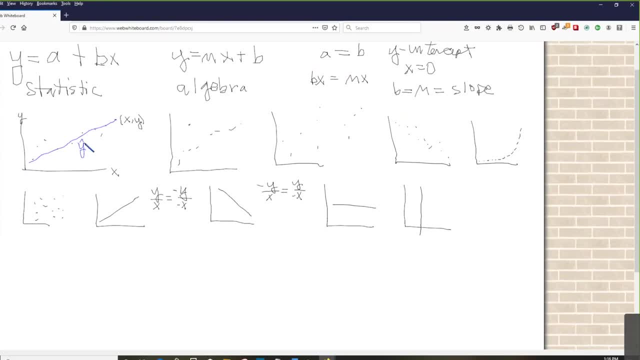 So the equation for this line- and we're going to do an example here pretty soon- is going to be: y hat, or, which is an estimated: y equals a plus bx, And we get this y hat, We calculate this. So this point- let's say this point here- that's going to be like y1, x1. 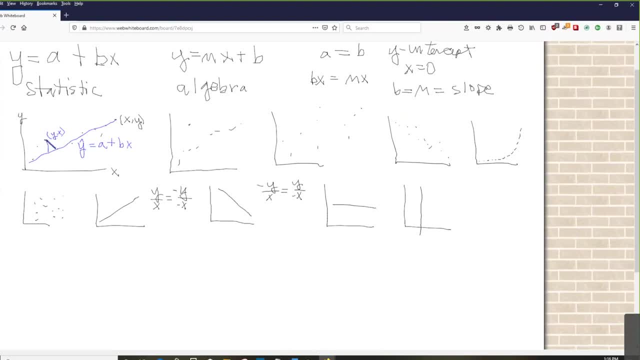 Then this point: this difference between where that point is and where that line is is going to be the difference between y1 and y hat, And we can calculate All the errors and we'll go into this more, but this is called when I sum. 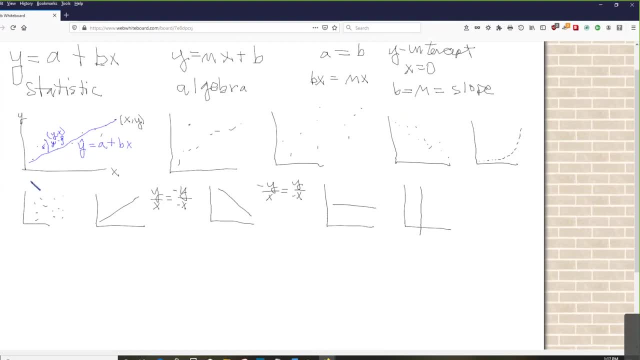 this is called an epsilon and I get my. where is it? the sum? so the sum of the squared errors is going to be the summation of all of these Y minus the estimated. So it's going to be the point minus the point on the line squared sum, and that's going to be kind. 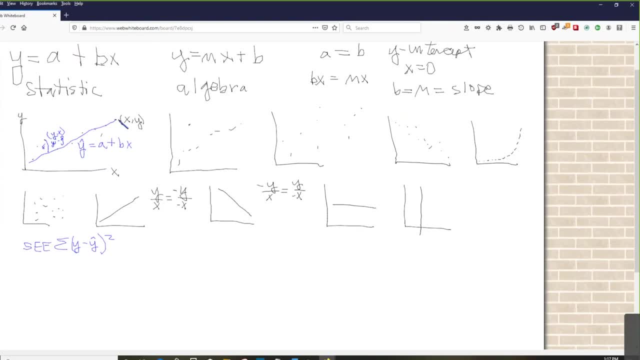 of all of the errors and this line, this best fit line, is going to want to minimize that error as close, as much as possible. So that's just really brief explanation And we'll go into that more detail on how all of this equation can be. 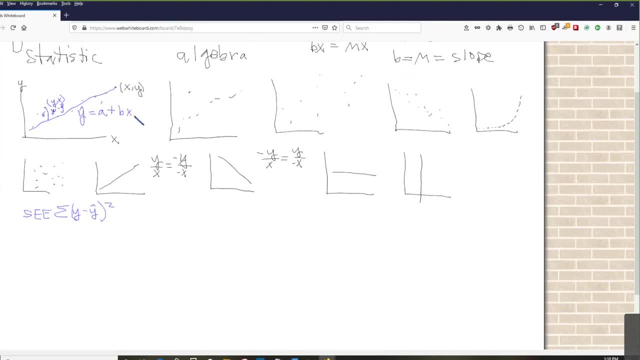 how this equation is derived. You can go to the Khan Academy of Statistics videos and they have some videos on line regression and they will go through all the steps of how that line is calculated. But in order for you to solve the problems with your assignment, 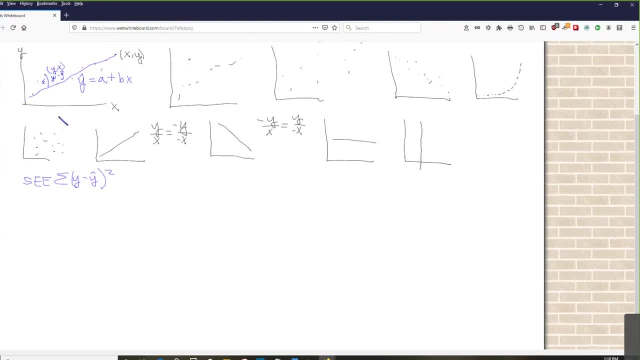 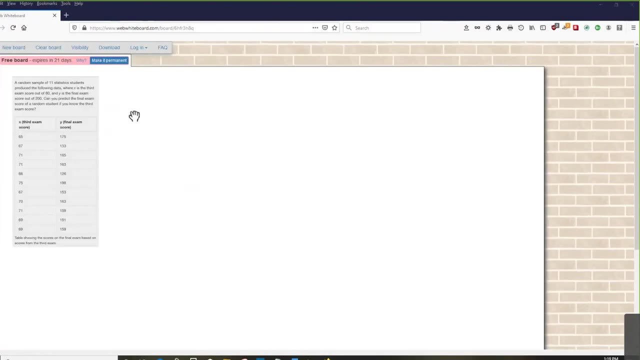 you don't need to know that process. So I'm going to just go ahead and skip that part and you can look at that if you want. So let's go ahead and do an example. So if we have a random sample of 11 statistics, students produce the following data: 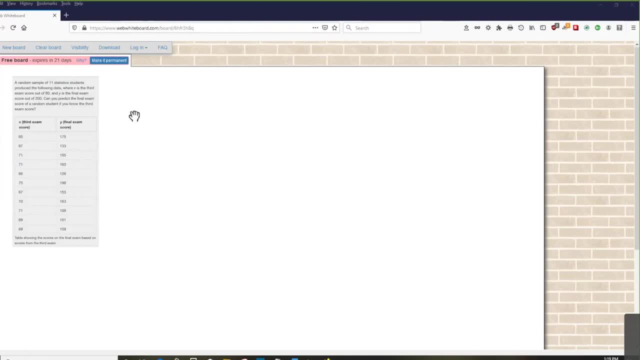 where X is the third exam score out of 80, and Y is the final score. final exam score out of 200.. We want to know: can you predict the final exam score of a random student if you know the third exam score? 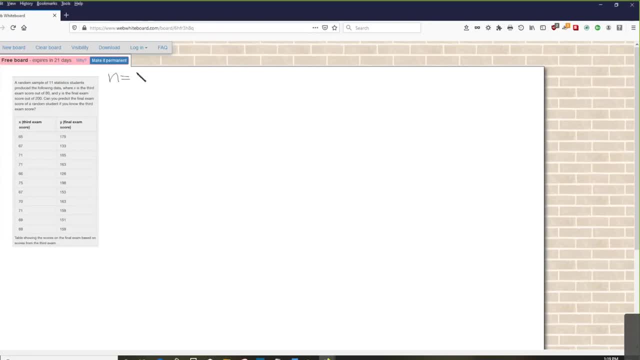 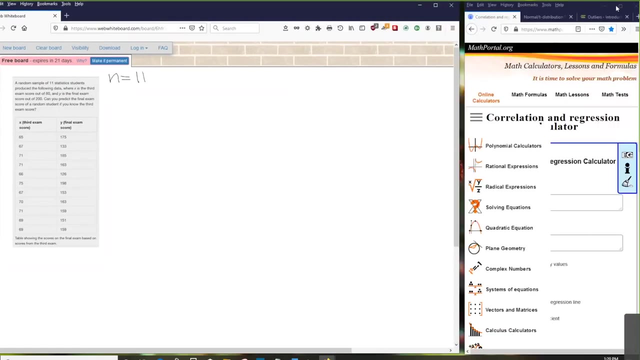 So let's write down what do we know We have N is going to equal 11 students, and then we've got our X's and Y's. So for, in order to solve this, we're going to need our, we're going to need 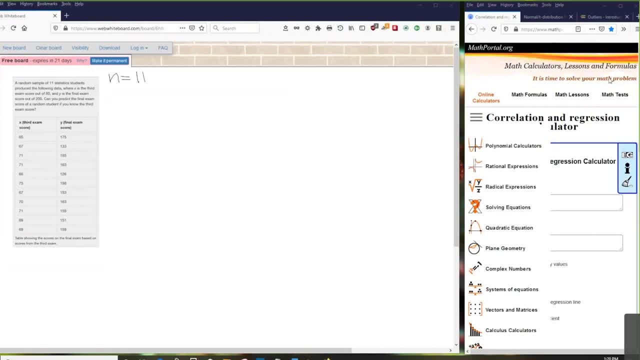 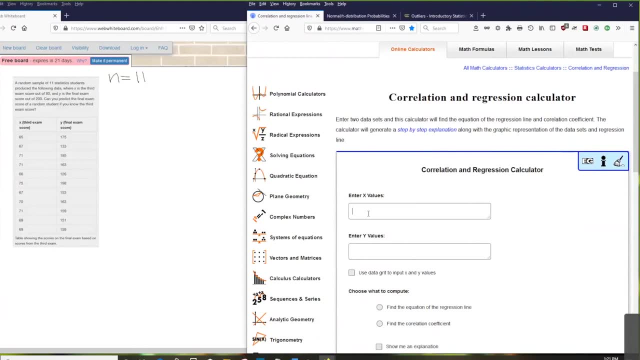 to use a regression algorithm And it's going to be a regression calculator. So from my data I'm going to go ahead and put in my values And with this, you just need to have a space in between each of these numbers. 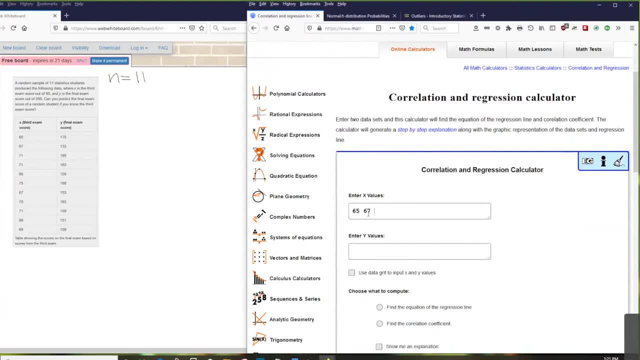 So I've got 65,, 67,, 71,, 71,, 56,, 75,, 67,, 70.. And then I've got my values. I'm going to go ahead and put in my values. So I've got 65, 67,, 71,, 71,, 56,, 75,, 67,, 70. 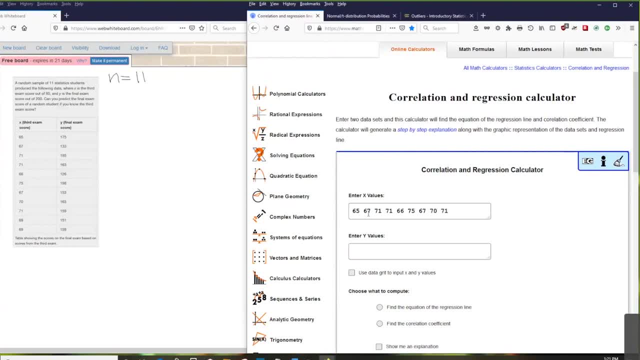 And then I've got my values, And then I've got my values 71,, 69,, 69,, and then I'm also going to do the Y values 175,, 133,, 185,, 163,, 126,, 198,, 153,, 165,. 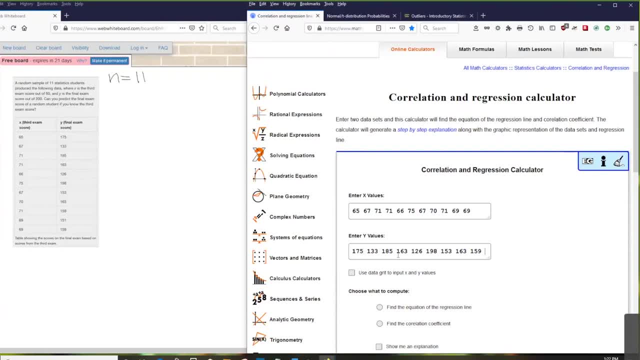 153, 159,, 151, 159,. okay, so these are. so our X values are the third exam score and then our Y values are the final exam score, and then we're going to use this calculator and then we're going to use this calculator. 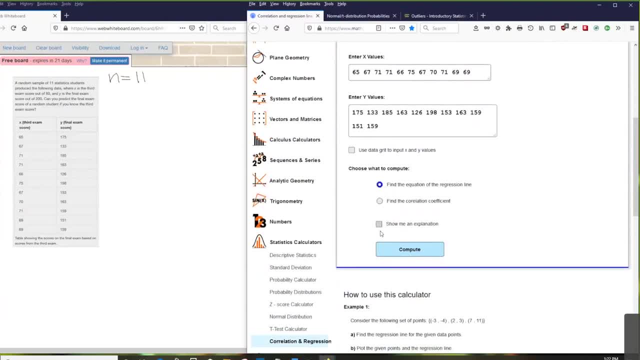 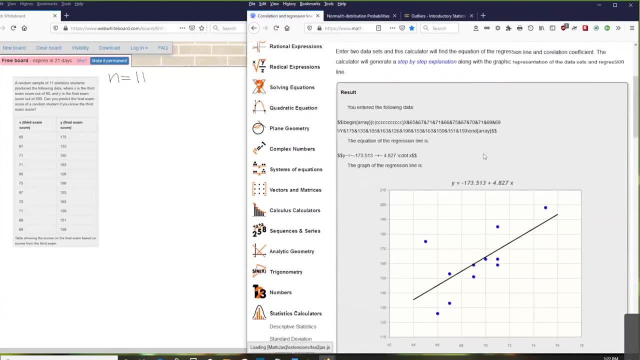 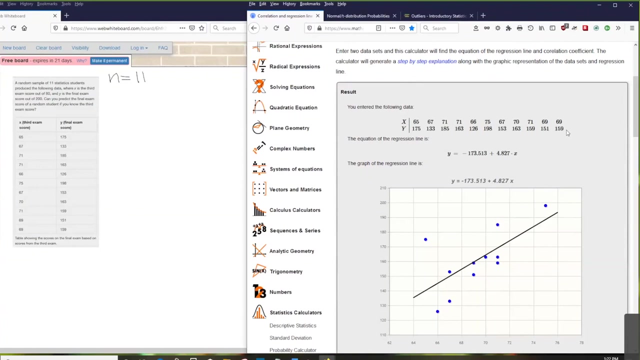 to find the equation of the regression line, and then I'm also going to click here. with this calculator, you can also show an explanation. So this online calculator is going to give me, show me, all my data. it's going to give me the equation of the regression line. 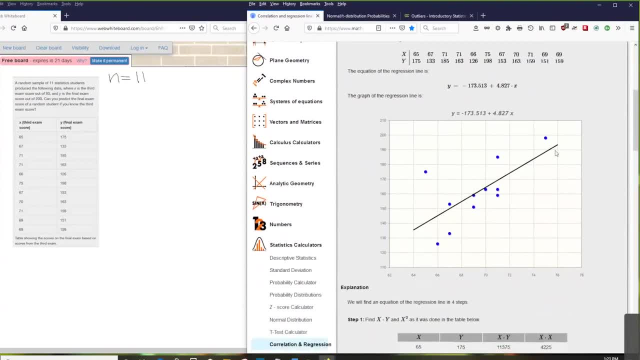 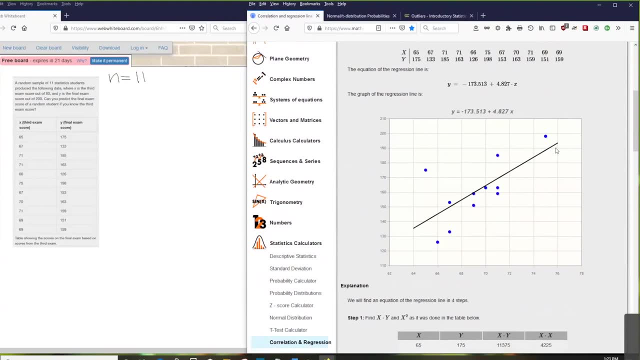 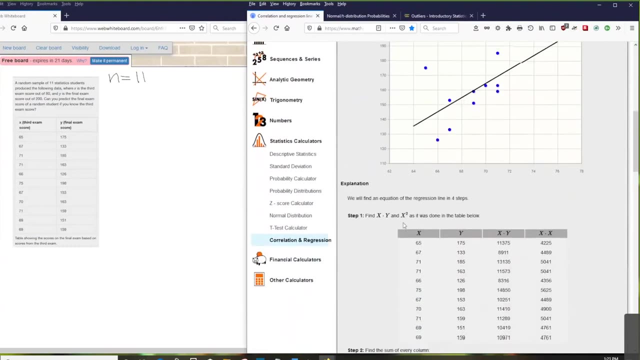 and it's also going to graph it. so, this straight line, so it's graphed, all of my points, and then it's also going to give me the straight line which is this best fit line, and then here it's also going to show me how all of this was figured out. 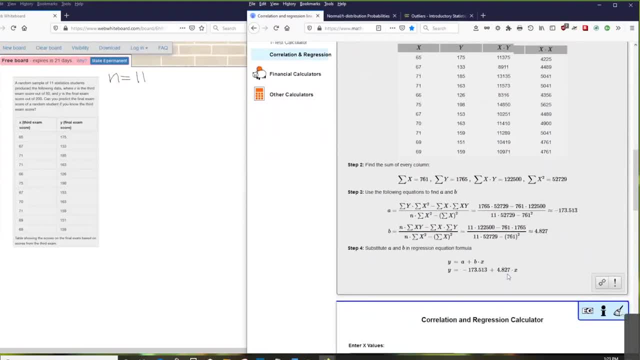 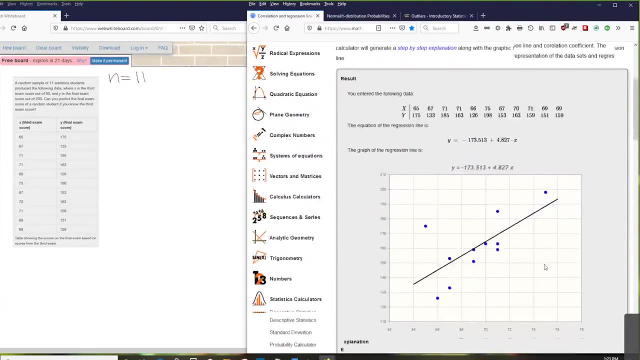 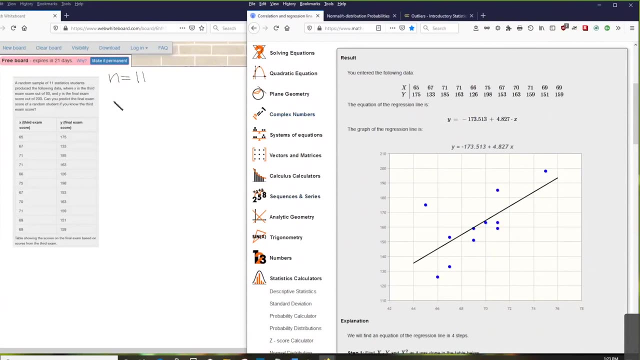 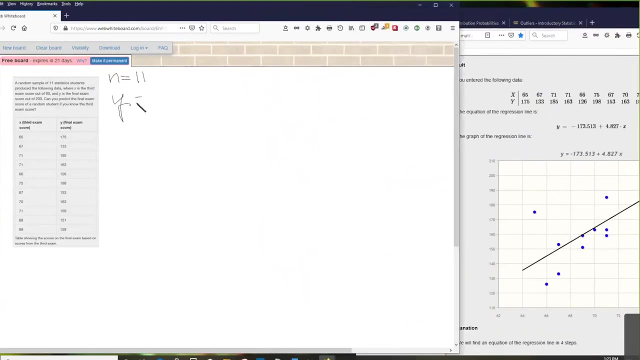 just so that you can see where did this, where did this information come from? okay, so so using our calculator, we were able to calculate, okay, that our equation, the best fit line, is minus 173.513, plus 4.83.. 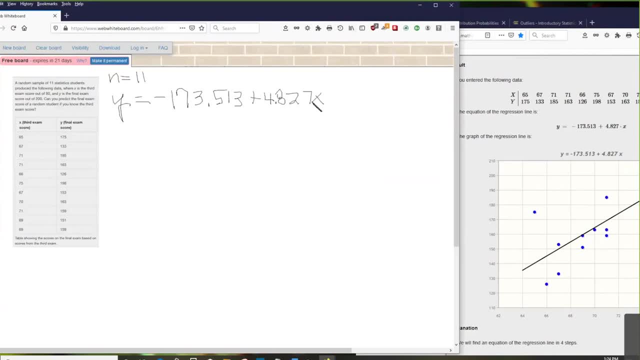 Okay so. so, using our calculator, we were able to calculate that our equation the best fit line is minus 173.513, plus 4.83.. Okay so. so, using our calculator, we were able to calculate that our equation the best fit line is minus 173.513,. 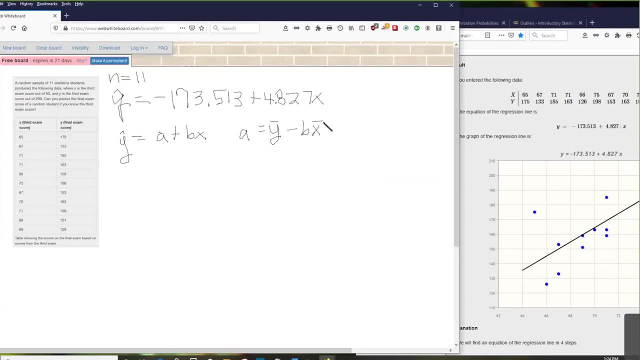 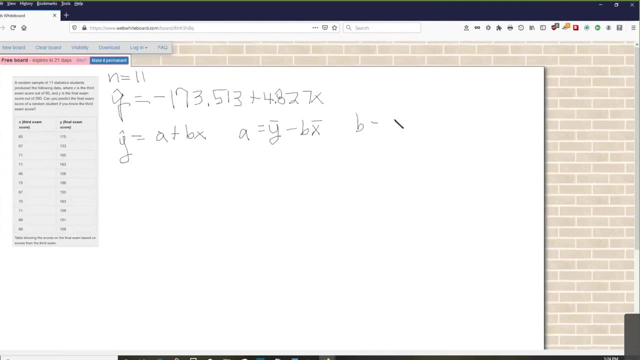 plus 4.83.. Okay so, so, using our calculator, we were able to calculate that our equation, the best fit line, is minus 173.513, B times the mean of X. B is going to equal the summation of X minus the mean. 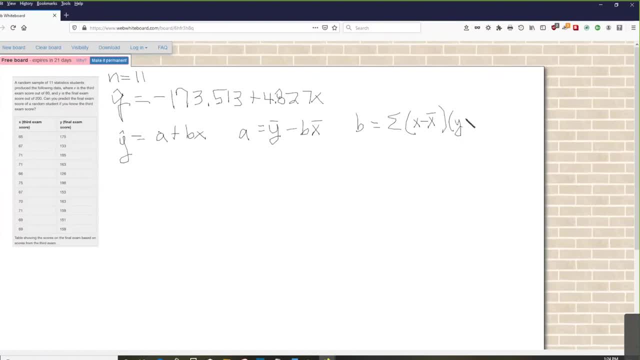 of X times Y minus the mean of Y, all divided by the summation of X minus the mean of X, quantity squared, And the best fit line is always going to pass through the point. it's always going to pass through the point of the mean of X and the mean of Y. 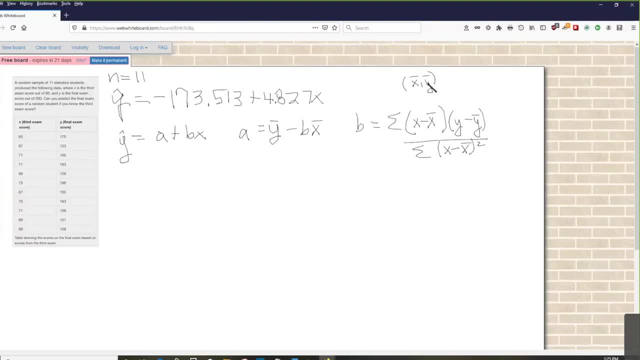 Another way that you can write the slope. the slope can also be written in the form of R, which is the correlation coefficient which we'll look at next times: the standard value of X, So the standard deviation of Y divided by the standard deviation of X. 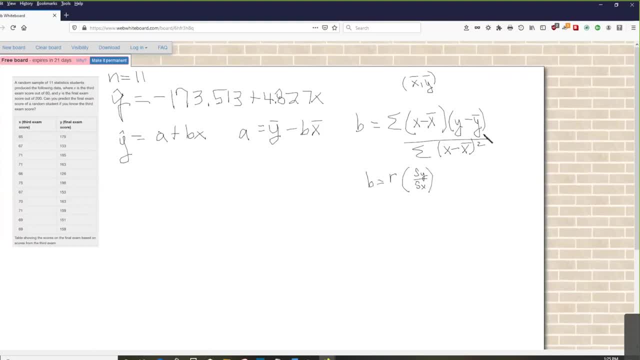 And it's important to know what these formulas are. but you're going to use your calculators in order to solve it, And if you had the T184 calculator and you plugged that in, I'll show you what that looks like. All right? 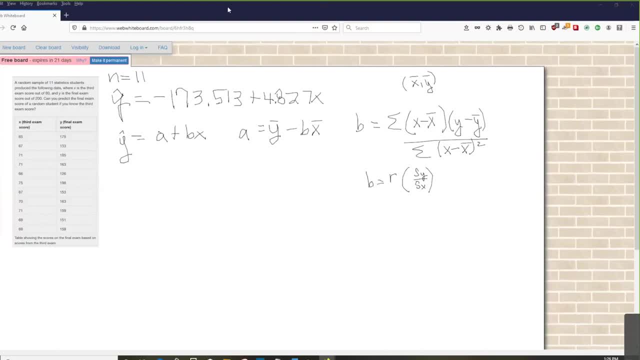 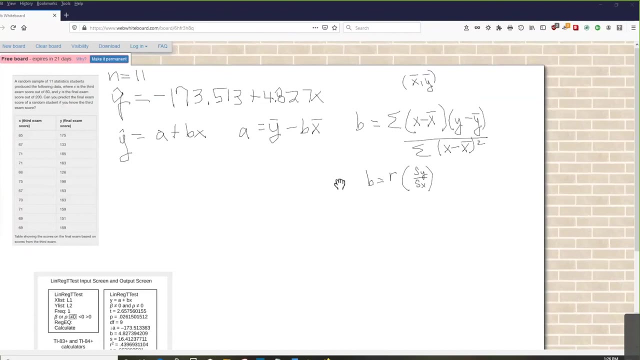 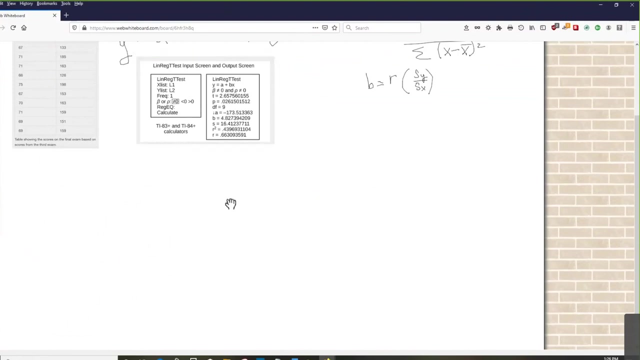 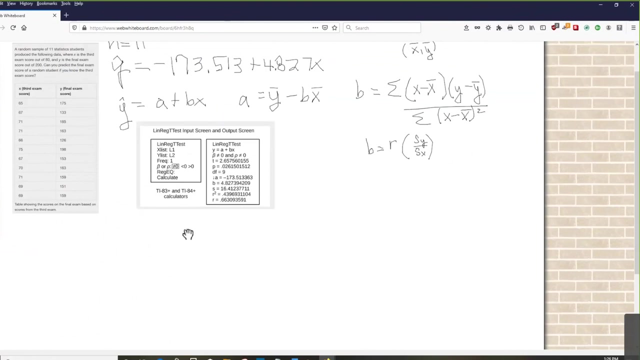 So let's see, And the book, if you have that calculator, the book will walk you through the steps of how to use that calculator. But you can see from This screen that it gives us once again, it gives us the equation for Y. 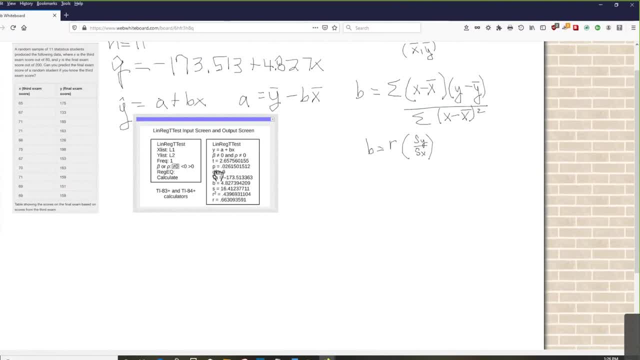 And it will give you your. let's see. so your in addition to your equation right here. so it's going to give you your A and your B. Okay, So you can see the calculator. we got real similar results. 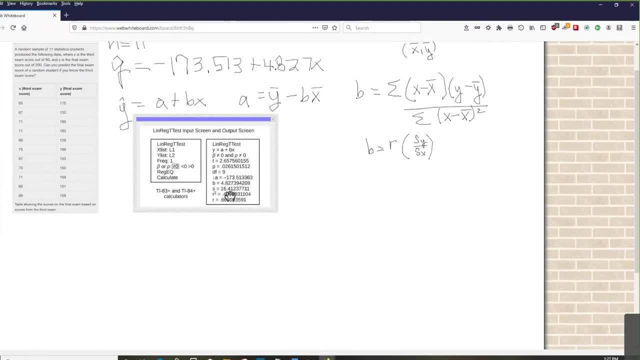 This one is also going to give you S, which is your standard deviation, And it's going to give you your R, which is your correlation coefficient, And you can calculate the. you can calculate these numbers other in other ways, But I wanted you also to be able to see what it looks like on the calculator. 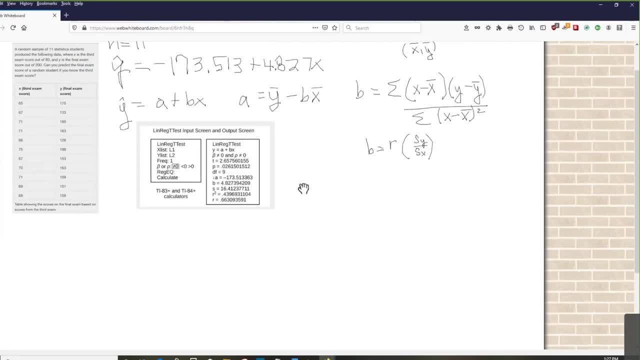 And if you That software- The link that I showed you, I sent you guys last time- they the Texas Instrument- you can download that software for this calculator and get a free 90-day trial. So for some of this ladder stuff, if you haven't already done that, 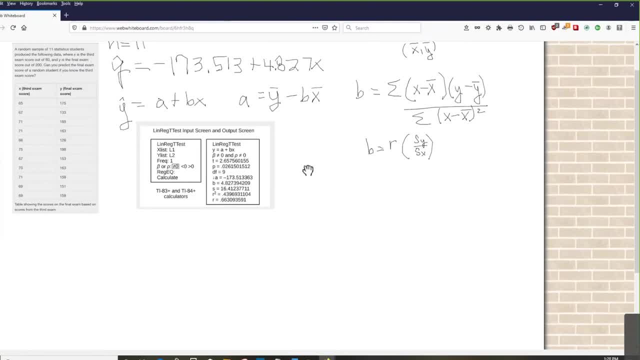 and you don't have the T184 calculator. you might want to do that, Just because I'm seeing some variability as far as calculating things by hand versus what's showing up with the calculator. So I'm going to go ahead and show you how to do that. 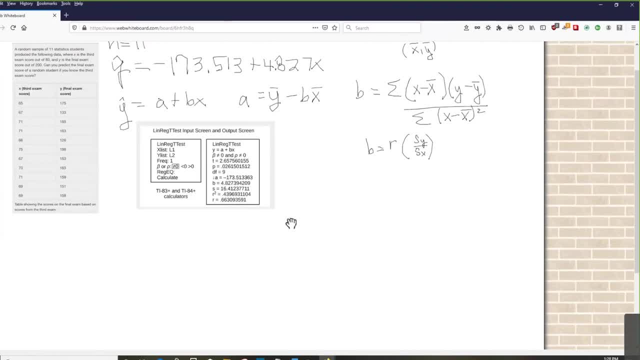 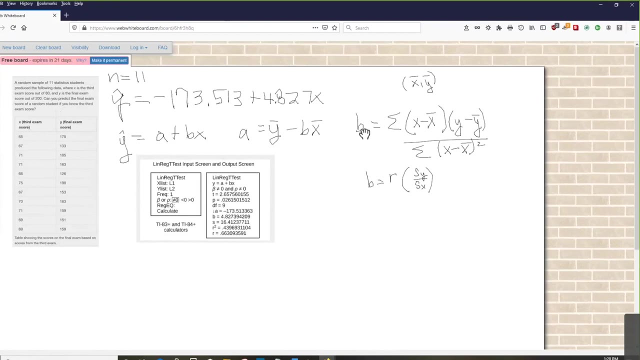 So I'm going to go ahead and show you how to do that, Okay, So so we use our online regression calculator to get our equation based on our data, to get our equation for the line, because that will solve for our A and our B values. 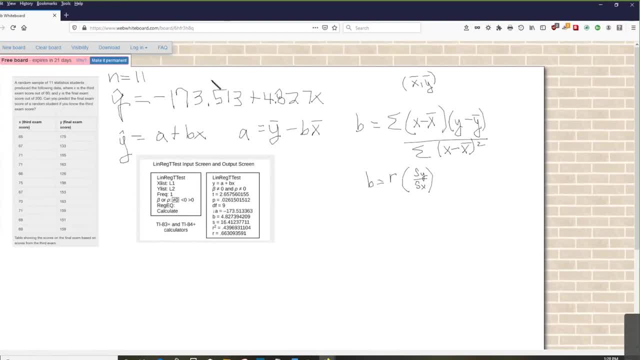 So this is my A and this is B, So remember that the formula is: the Y equals A plus BX. okay, So the way that we would interpret this, so the B or full B, tells us how Y changes for every X. 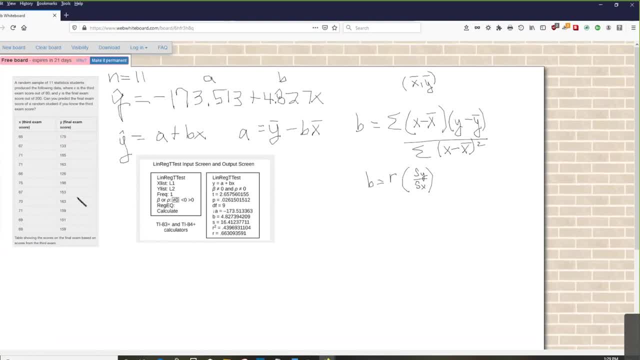 So for this particular exam, we got a B. our B is going to be equaling to 4.827,, which we could round to being 4.83, and that all that's saying is for a one-point increase. on the third exam, which is our X values, then we would expect the final exam. 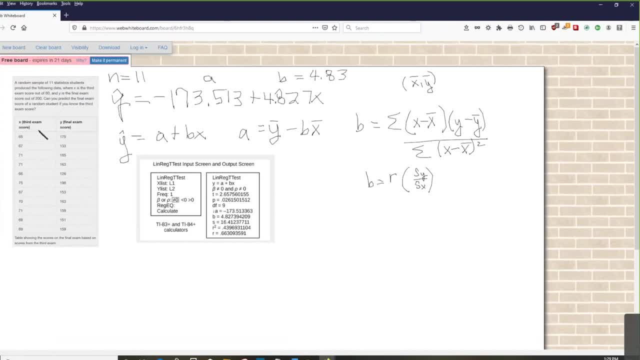 the points to increase by 4.83.. So now let's go ahead and show you how to do that Now. the process of fitting the best fit line is called linear regression. It's based on the assumption that data is scattered about a straight line. 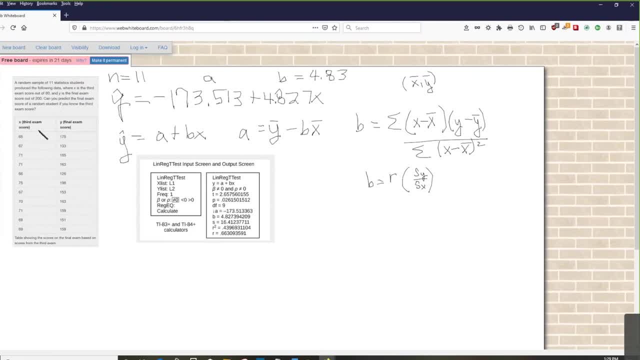 The best fit line is the line where the sum of the squared errors is minimized, And that's what I was showing before, where the distance between the data points and the line you want both to be as small as possible. The best fit line is the line where the sum of the squared errors is minimized. 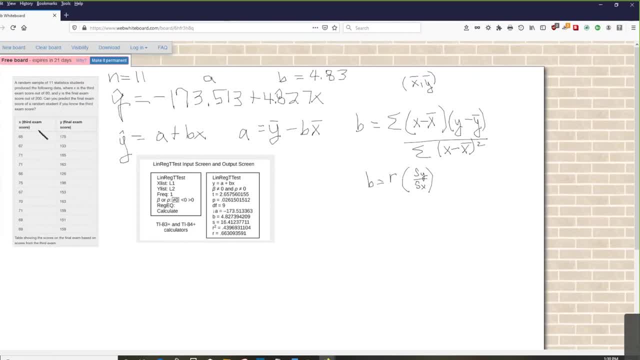 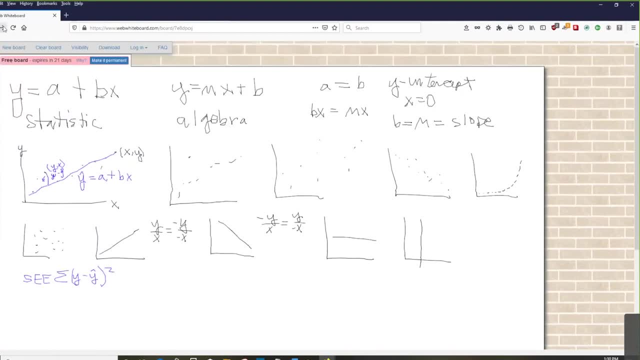 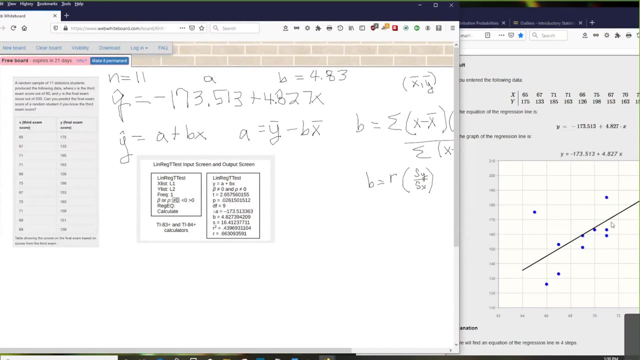 line is called the least squares regression line and that says, if we look at, let's go back. so if we look at our calculator, so this line right here, that is called your best fit line. it is also called the least squares regression line and the sum of the squared errors is the sum of the squared distance between the. 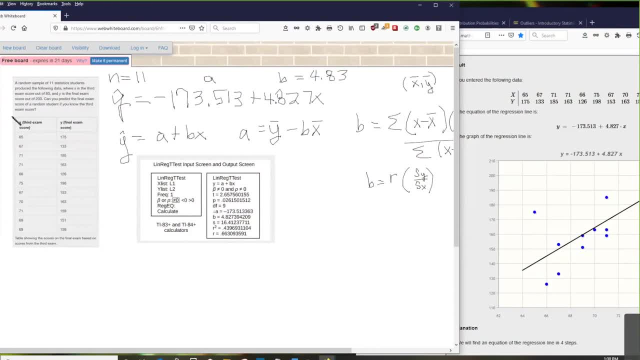 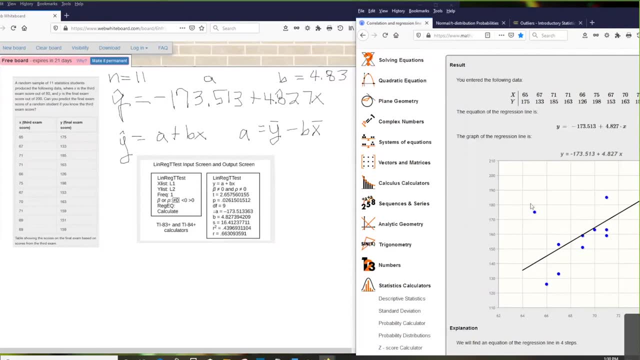 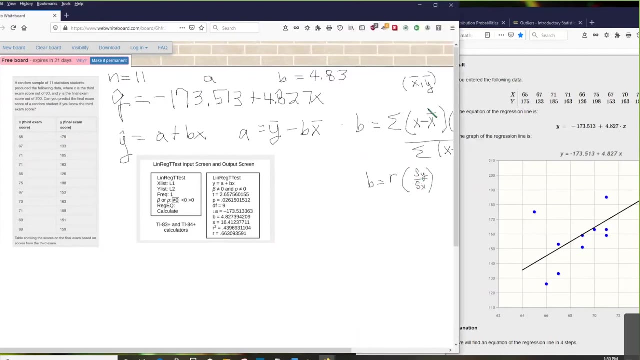 actual data point and the line of best fit. so that's what we talked about right through here. this line, this distance between these two points squared and added together, is going to get through some of the squared errors. so now the next thing that we need to calculate is we want to calculate this R, which is the 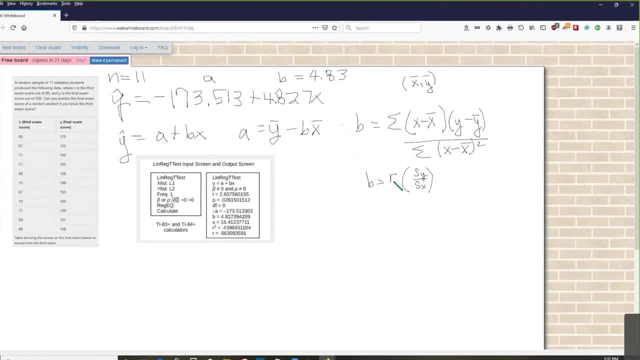 correlation coefficient, because that tells us that provides a measure of the strength and direction of the line of best fit. so that's what we talked about here last week. so now, remember, we're going to use the equation that spooned out this formula for the length of the slit, and then we're going to use this: 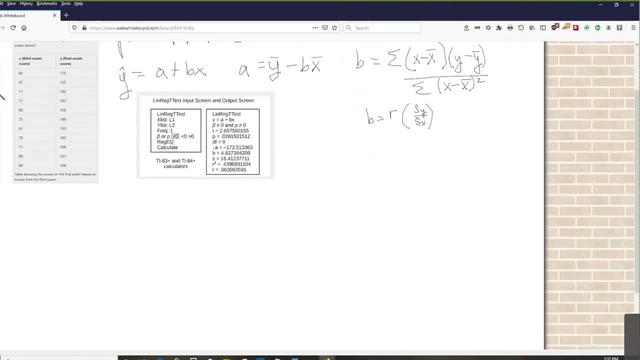 time to calculate the length of the slit, and then this is going to be the association between the dependent X values and the dependent Y value, and this is also something that our online calculator will calculate. so the formula for R is going to be n, which is the number of data points that we have times the summation of X, times Y, times y, times the percent illusion of that measure. 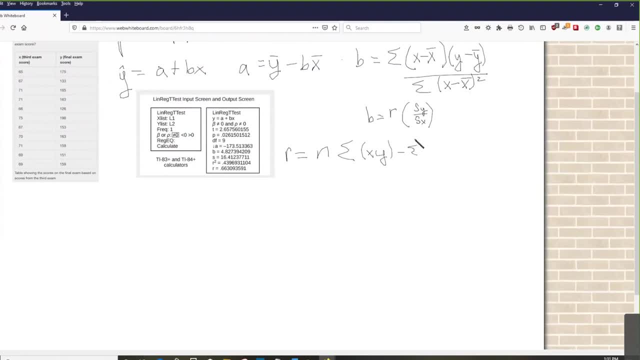 Y minus the summation of X times the summation of Y all divided by the square root of N. summation of X squared minus summation of X squared minus- excuse me- times N. summation Y squared minus the summation Y squared. Now our okay, so let's go ahead and go back to our calculator. 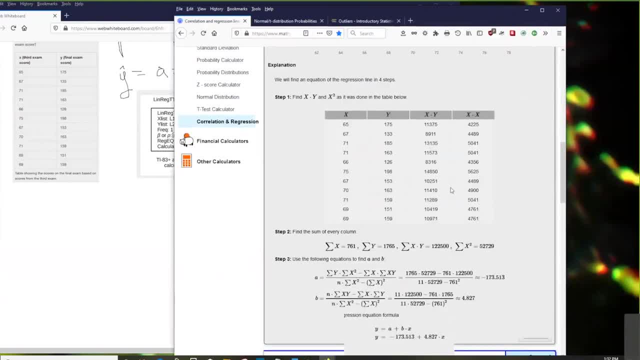 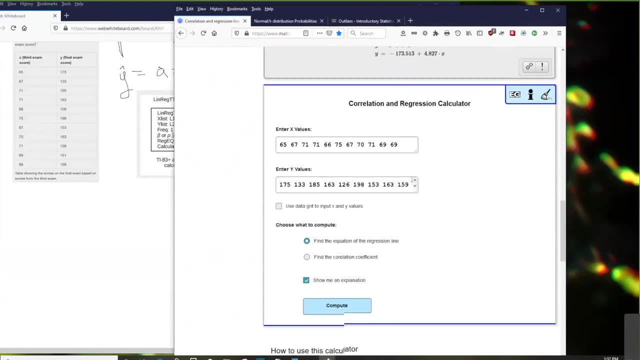 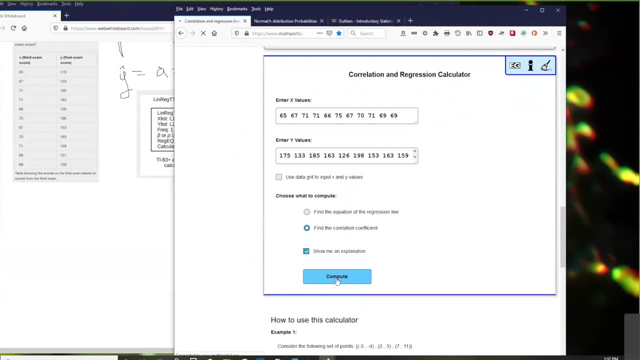 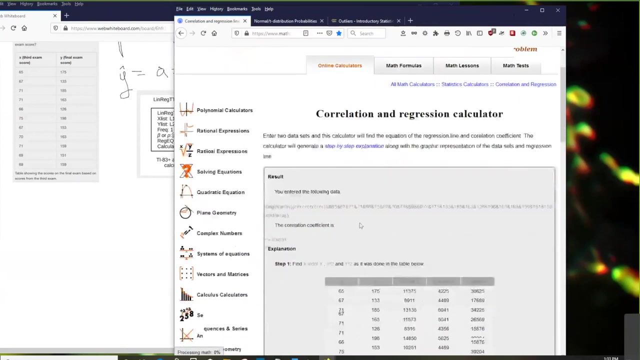 So this same calculator will also. so it saved all of our data points. So once we get our equation of the line, then we can go and switch it to find the correlation coefficient. So once again, it's going to show us our data, it's going to give us our correlation coefficient. 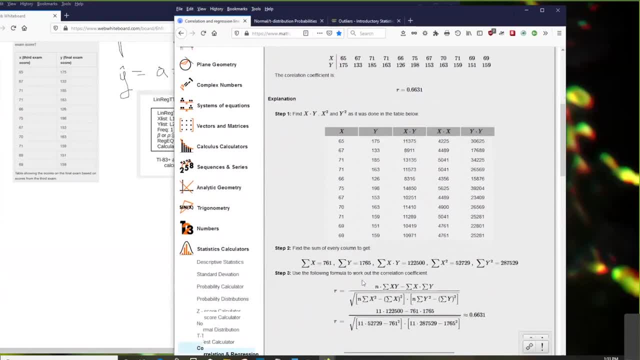 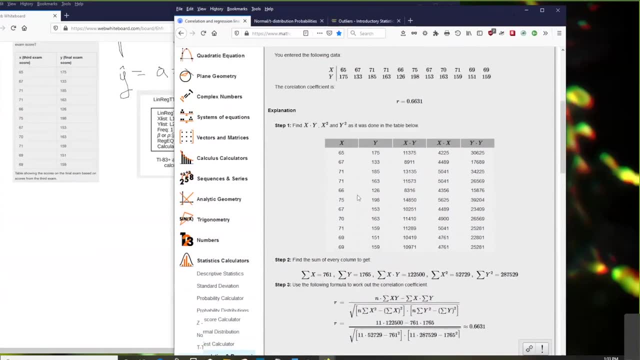 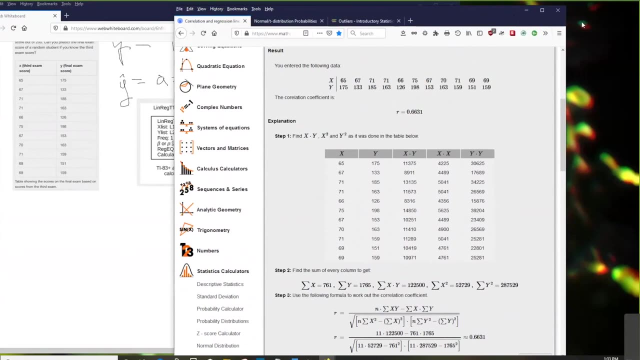 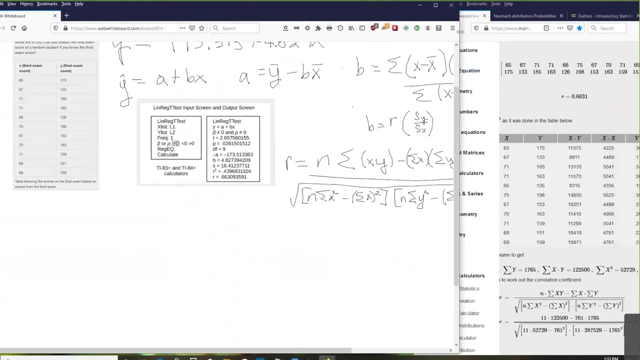 and it's going to also show how everything was calculated, And you can keep this second half of showing the steps if you want, or you can do it. you can still do the calculation without that. Okay, So this is giving us a correlation coefficient of 0.6631. 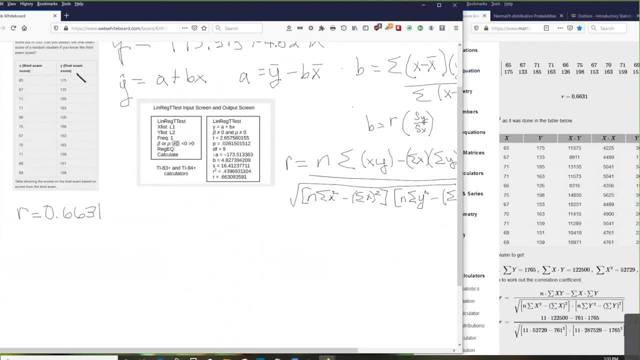 for our data using these two exams. So the few things about R. R is always going to be between minus Y and the square root of X. Thank you, Thanks, R. All right, Thank you, Thanks, guys. Thank you. 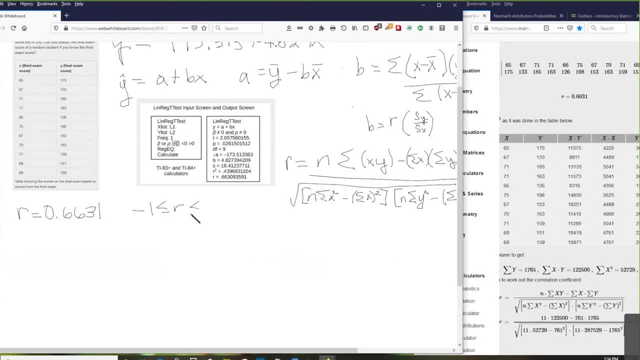 Thank you, Thanks, Thanks guys, Thanks, Thanks. one and a positive one. So if r is close, the closer the r is to either a negative one or a minus one. then that's going to show a stronger relationship. 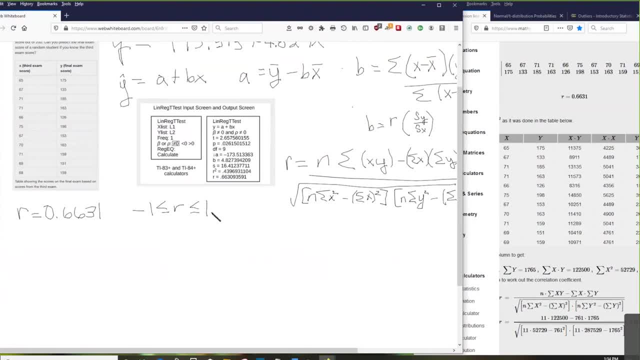 If it's going close to a one. if r equals one, that's a perfect positive correlation. If r equals a negative one, that's a perfect negative correlation. If r equals zero, there's no correlation. So the stronger two plus or minus. so if I'm on a graph, 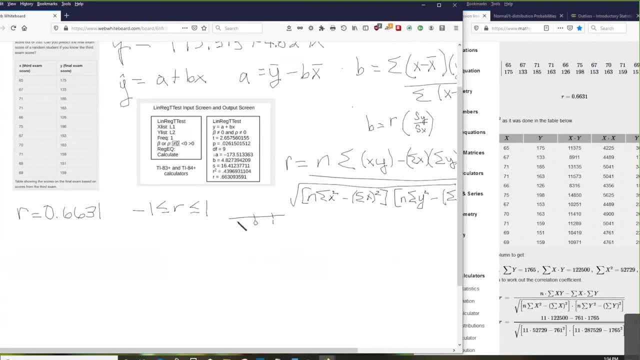 and here is zero, here's one, here's minus one. this is going to be zero relationship. So zero relationship to this is going to be real strong, And this is going to be So when it gets close to the one or the minus one. 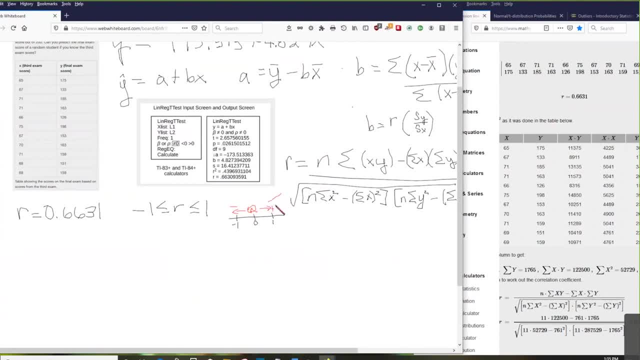 it's going to be real strong. And a positive just means it's going to go to the right, Negative means it's going to go to the left and that's the slope of the line And the sign of whatever the sign the coefficient is. 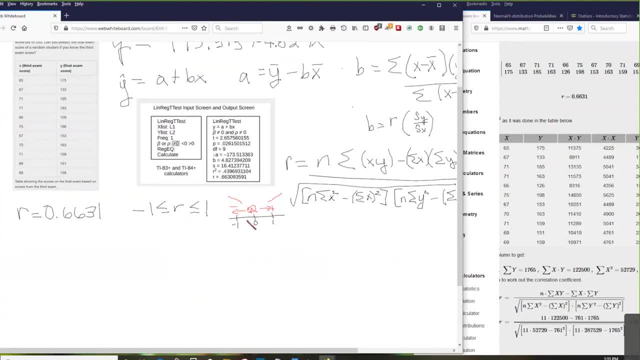 that's always going to be the same sign as your slope. So if I have a negative r, we're going to also have a negative b or a negative slope And a negative correlation. So now we have the coefficient determination, which is your r squared is usually: 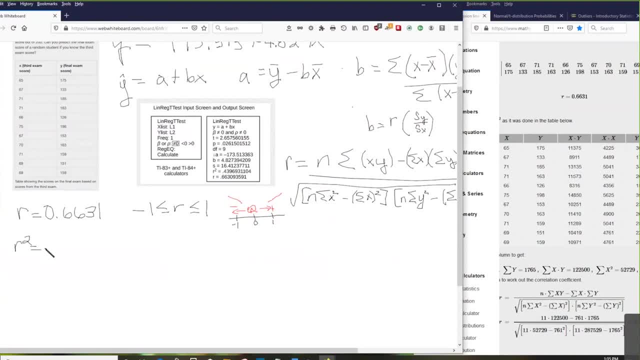 expressed as a percentage. So the percentage, and it's the percentage of variation in y that can be explained by variation in x, using the best fit line, And one minus r squared. So this is so, this we can, so this is going to be. 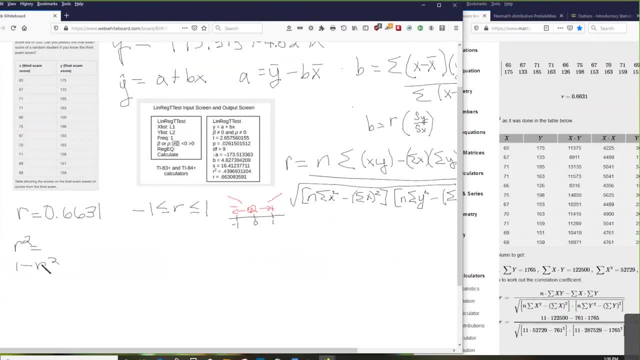 like it can be explained. And then the one minus r squared is also going to be listed as a percentage and it's the variation not explained Or it's the scattering of the observed points. So for this particular problem, if I have an r of 0.6631,, 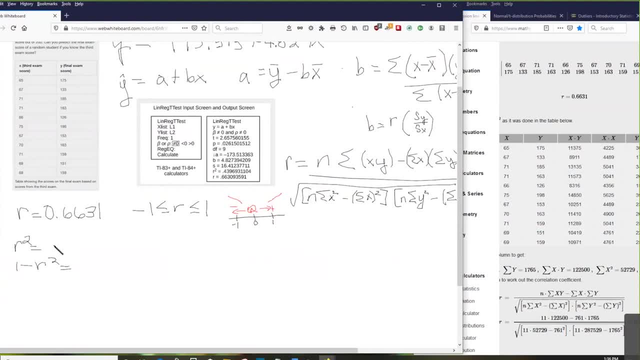 then my r squared. I'm going to square that and that's going to give me a calculation of 0.4397016.. So that means that I'm going to be able to calculate, you know, as a percentage my r squared is going to be about 44%. 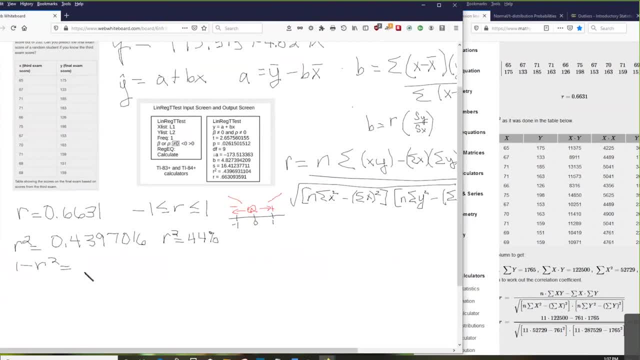 My one minus r squared is going to give me- I'm just going to take one minus that number and that's going to give me a 0.5602983.. So that means, once again, I'm going to say this as a percentage- 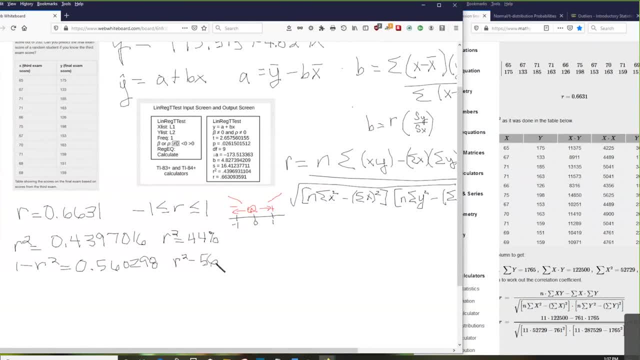 So this is going to give me my r squared is going to be about 56%, And then, if you'll notice on the calculator results, it gave you both r, which was the correlation coefficient, and the r squared, which is your coefficient of determination. 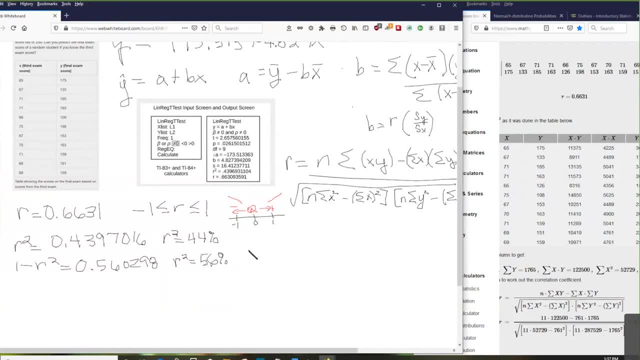 And then the way that we interpret this is. we say approximately. so for this particular set of data, we would say approximately 44% of the variations in the final exam grades can be explained by the variation in the grades on the third exam using the best fit regression lines. 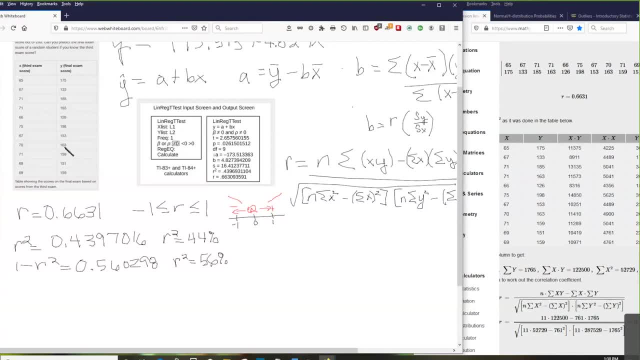 Therefore, approximately 56%, which is our one minus r squared 56%- of the variations in the final exam grades cannot be explained by the changes in our Diesel kannne, in our similar model, explained by the variation in the grades on the third exam using the best fit regression line. 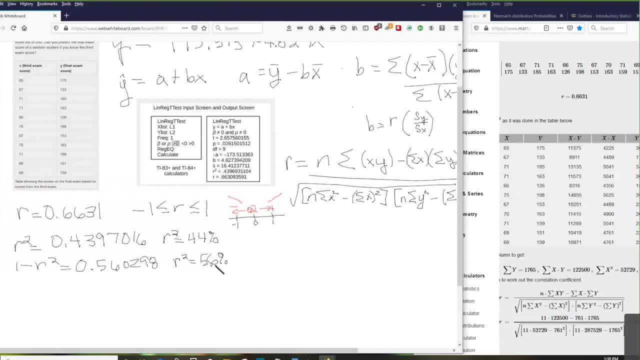 And so that is how this explains the point scattering on our data which we saw before. OK, Any questions so far? OK, The next thing we want to do is we want to test the significance of the correlation coefficient to determine how strong or weak 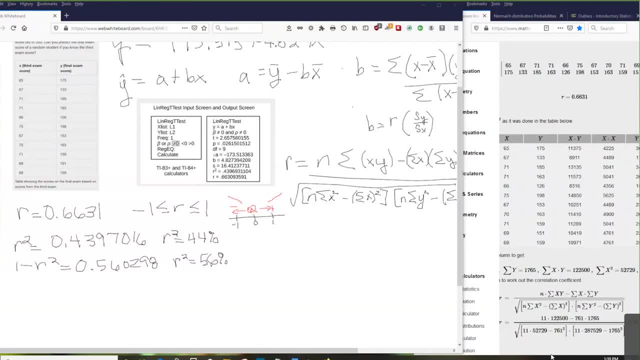 or whether or not there's a correlation. And with that we're going to use a hypothesis test to determine if the sample linear relationship is strong enough to model the population linear relationship. So so far we've just been working with the sample. 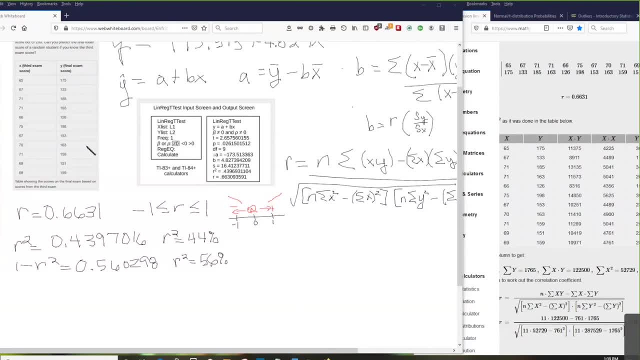 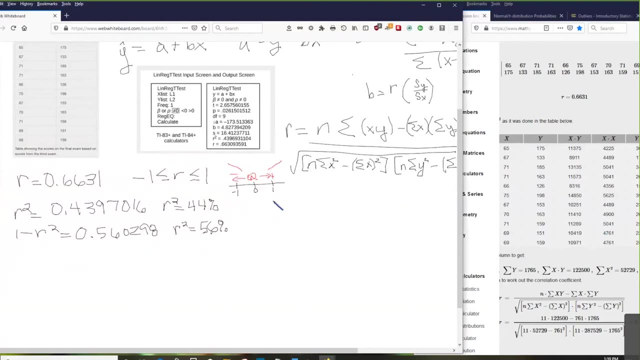 Now we want to do a test to determine: can this? is there a strong enough correlation to say that this applies beyond the sample to the population? So the way that we're going to do that is we're going to use the hypothesis testing that we've seen before, and what that is is our null hypothesis is going to 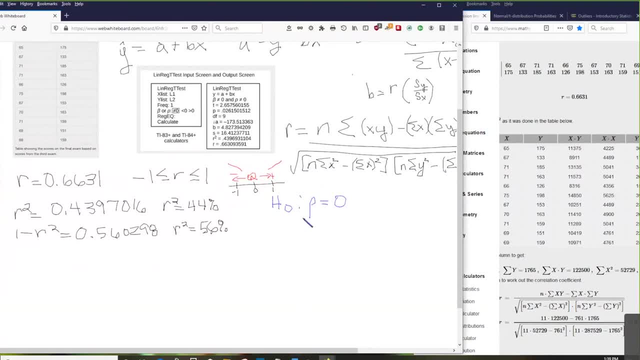 we're going to hypothesize that the population correlation coefficient, which is rho, is not significantly different from zero, which means there is not a significant linear relationship correlation between x and y in the population and we cannot use the regression line to model a linear relationship. 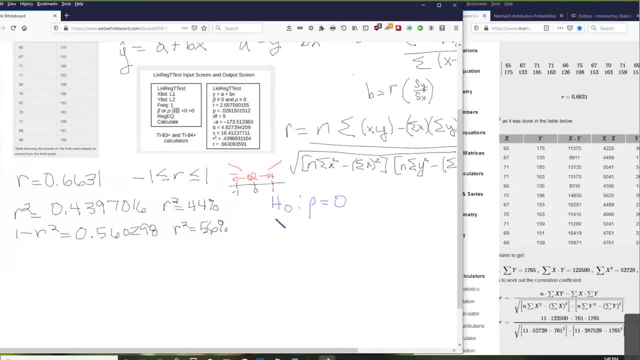 between x and y in the population. And we're going to put our alternative hypothesis to say that rho does not equal zero And that just says that the population correlation coefficient is significantly different from zero, which says there is a significant linear relationship or correlation between x and y in the population. 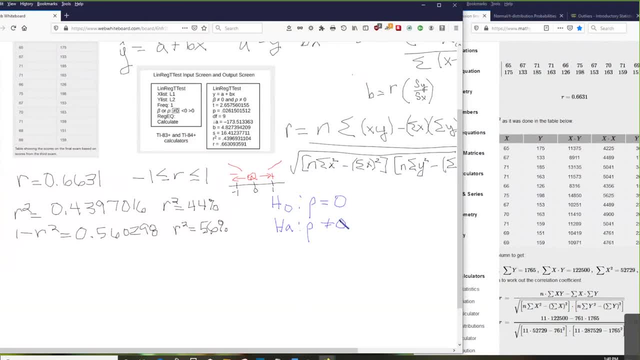 Therefore, we can use the regression line to model the linear relationship between x and y in the population. So we're going to continue using the same sample data with the test, and there's two ways that you can test this. So we're going to use the regression line. 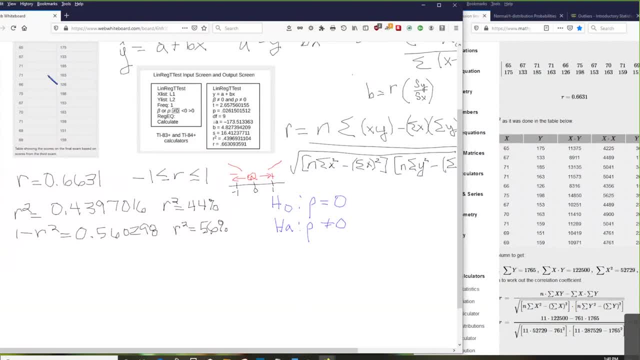 So we're going to use the regression line. So we're going to use the regression line And we're going to do this out. this hypothesis, The first one- is using a p-value method that's similar to what we've done before, and 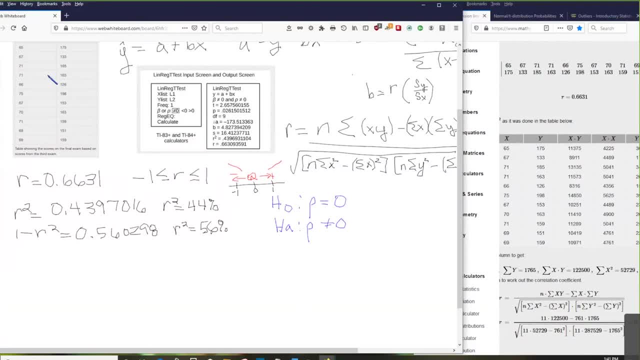 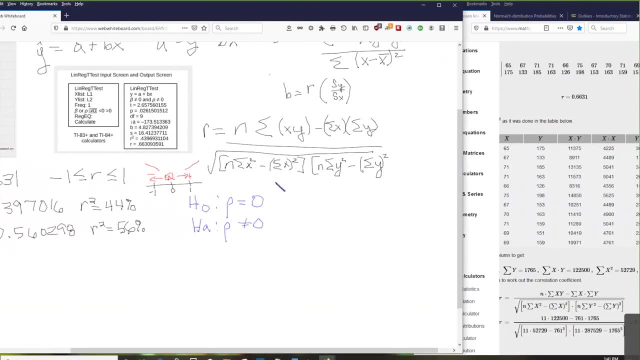 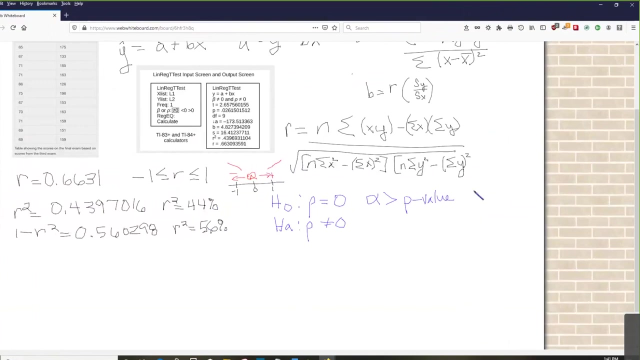 or the second method is using a table of critical value. So if, if our significance level is greater then the p-value, then we're going to reject the null hypothesis. So this is the same as what we've done before, is that the level of significance was greater. 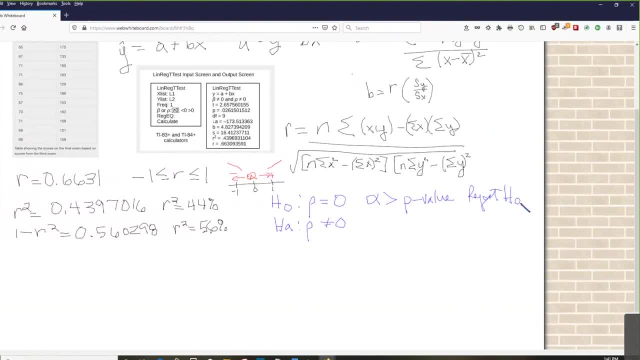 than our p-value, then we're going to reject the null hypothesis and say that the evidence supports the alternative. So this would be the conclusion would be: there is sufficient evidence to conclude that there is a significant linear relationship between x and y, because the correlation coefficient is significantly different from zero. 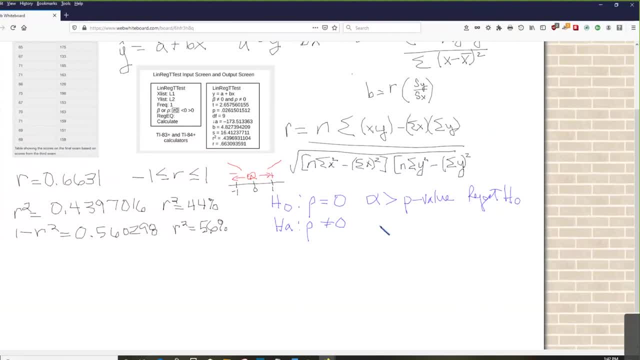 Now, if the p-value Is greater, so if the p-value, so if the level of significance is less than the p-value, or which we could write it either way. so if the level of significance is not greater, which means that it's less, then it means that we're not going to reject. 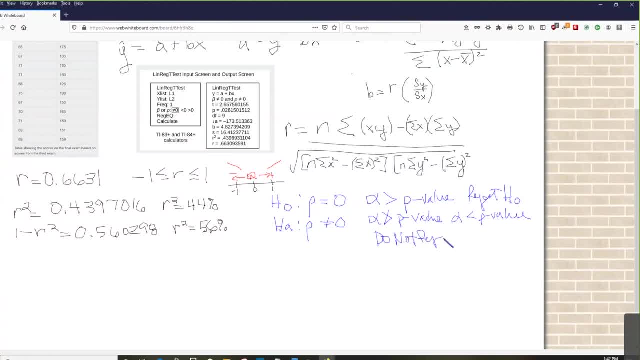 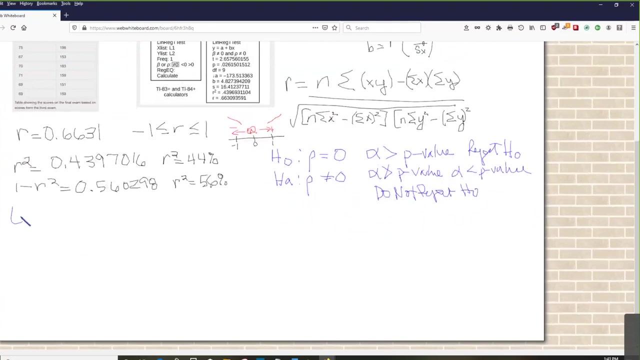 We do not reject the null hypothesis, and that means that there is insufficient evidence to conclude that there is a significant linear relationship between x and y, because the correlation coefficient is not significantly different from zero. Now, in order to do this, we are going to use the t-distribution. 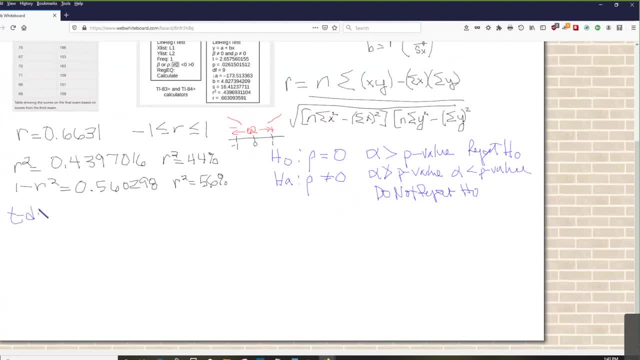 We're going to use our t-distribution. We're going to use our t-distribution calculator With degrees of freedom, With our degrees of freedom equaling n minus 2, and it's going to be n minus 2 instead of n minus 1, because we have two variables. 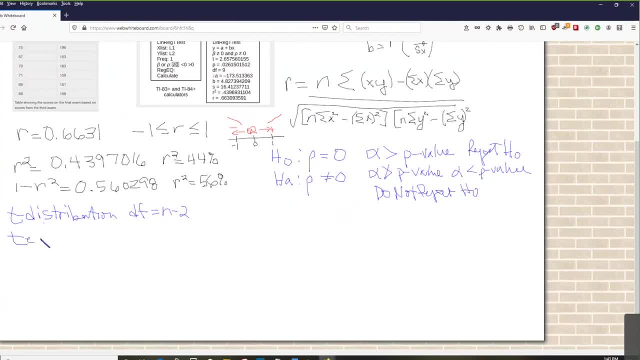 The test statistic that we're going to use. So our test statistic is going to have the formula of p equals r square root of n minus 2, divided by the square root of 1 minus r squared, And the p-value is going to be the error. 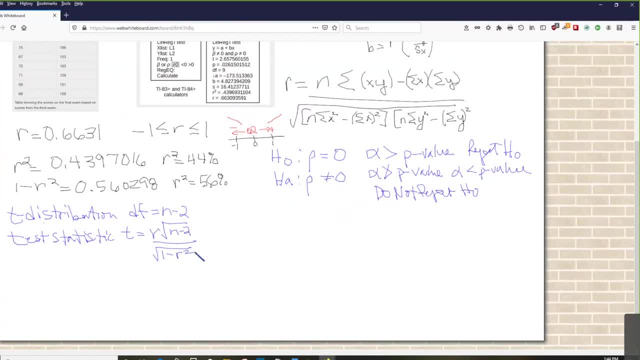 So we're going to use our t-distribution, So my t right here is going to equal the area of the two tails. So let's take a look at. we're going to continue on with this same sample, So let's solve, for that tells us that my degrees of freedom. 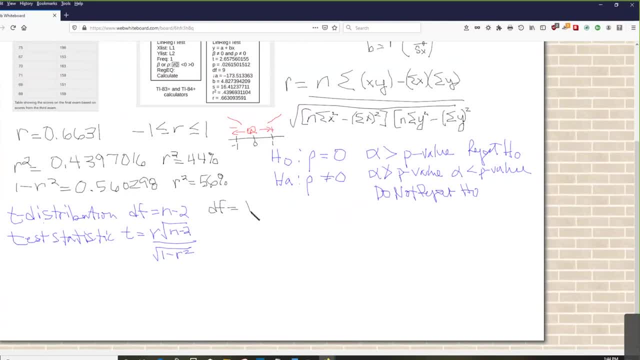 for this particular problem is going to be 11 minus 2, which is going to equal 9. to get my avenure of freedom, Here we go. I've got my r, which is going to be 66.6631, then I'm going to do the square root of n. 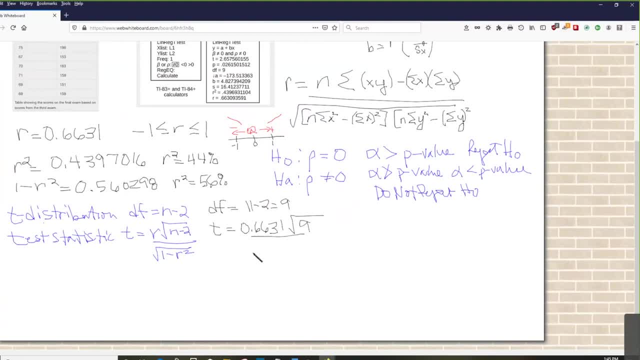 minus 2,, which is 9, and then I'm going to divide it by the square root of 1 minus r, squared, so that is going to be the square root of 0.560298, and then, when I do that calculation, I end up with a t score of 2.657601.. 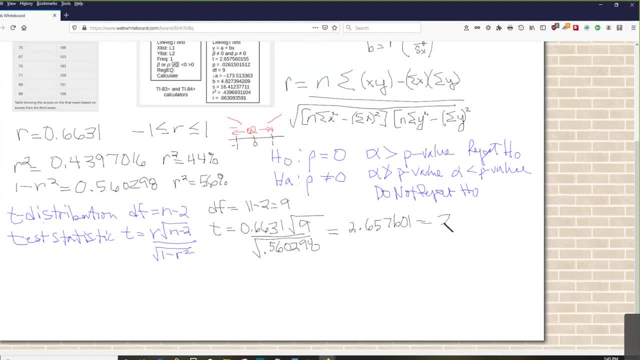 Okay. So now I'm going to want to find my t value of where x is greater than my t statistic, which is 2.658, so I'm going to plug that in, Okay. So now I'm going to want to find my t value of where x is greater than my t statistic. 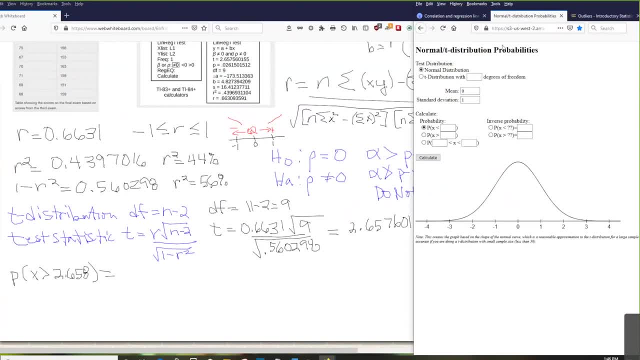 which is 2.658,, and then I'm going to plug that in. Okay, So now I'm going to want to find my t value of where x is greater than my t statistic, which is 1.658,, and then I'm going to plug that in. 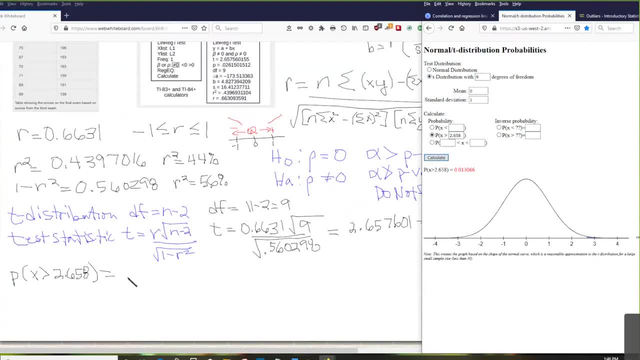 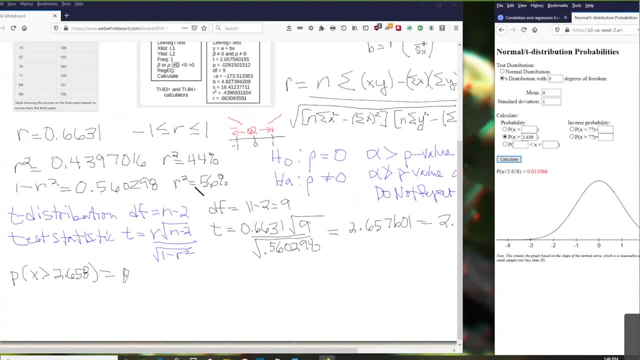 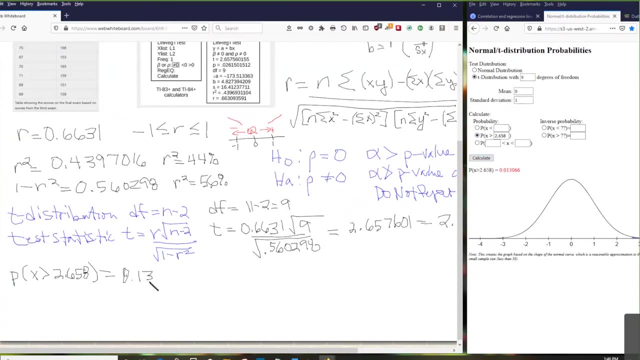 Okay, Okay. So that gave me a value of 0.13066.. And you want to remember, this is a two-tailed test because we're using the equal sign. So this is going to be half of my p-value. So, in order to get my p-value, I'm going to take this number, multiply it by 2.. 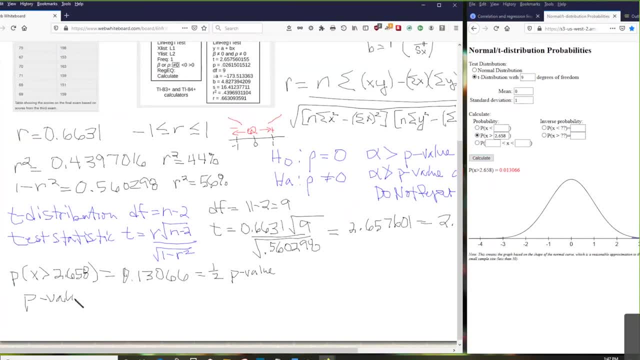 And that's going to give me a p-value of 0.026132,. okay, So now our critical value. Our critical value is going to be 0.05, because it wasn't stated, So we always assume if it's not directly given, then it's going to be 5%. 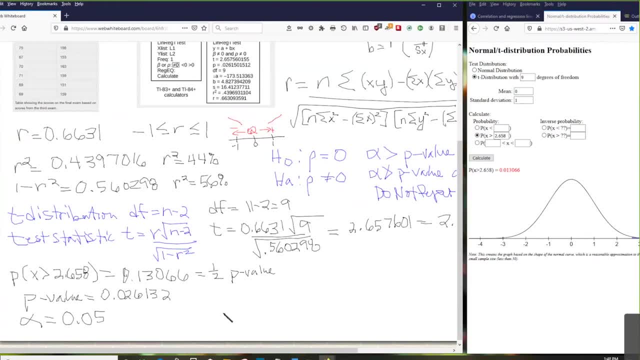 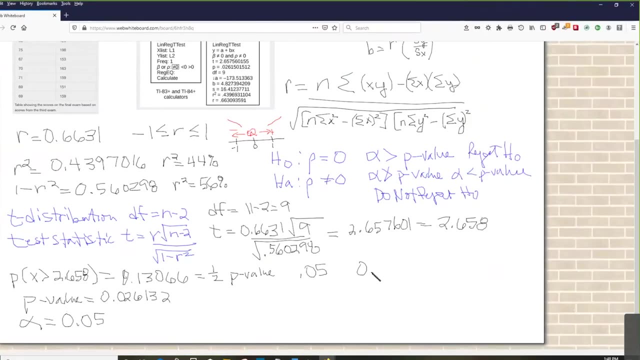 So now we're going to look at our rule. We're going to have our 0.05.. And 0.0261.. The 0.05 is greater, So our alpha is greater than our p-value. So that tells us we're going to reject the null hypothesis. 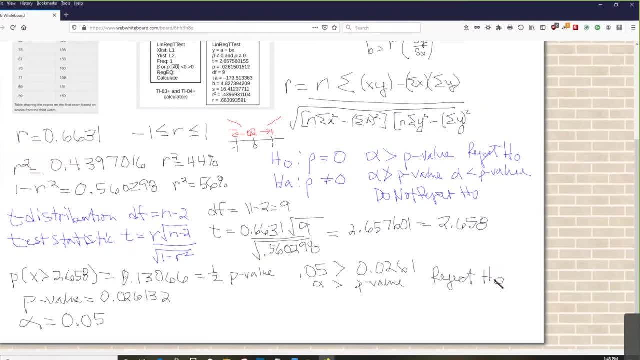 So that tells us that our conclusion is: there's sufficient evidence to conclude that there is a significant linear relationship between the third exam score, which are your Xs, and the final exam score, Y, because the correlation coefficient is significantly different from 0.. 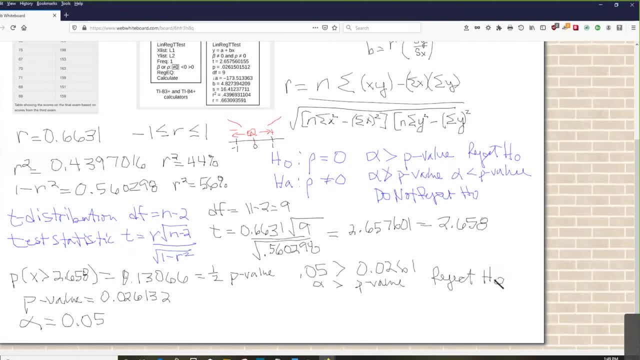 And because R is significant and the scatter plots show a linear trend that tells us that the regression line can be used to predict the final exam scores. okay, Any questions so far? Okay. Now, the second way that we can do that is using- so this is testing this out using the p-values. 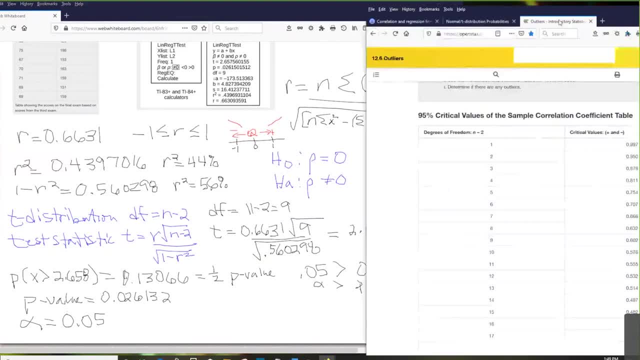 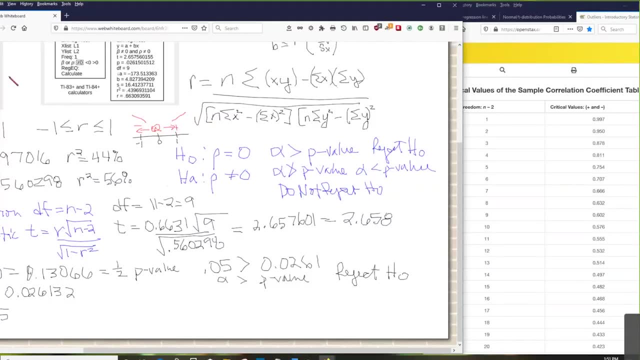 The other way that we can do that is to use a table of critical values. Okay, So what you're going to do, the way that you look at this is: you want to go to your. you're going to find your degrees of freedom. 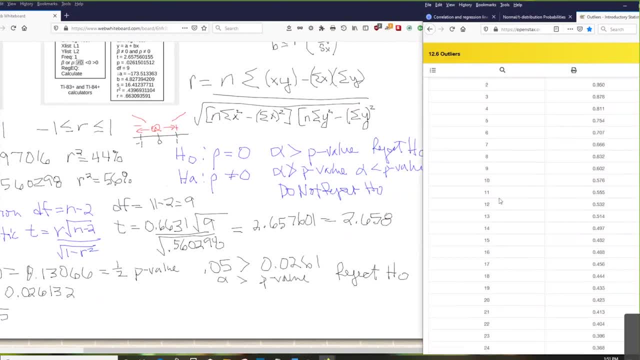 So in this case, our degrees of freedom here is 9.. And you're going to match it with the critical value, So this is giving us the critical value of 0.062.. So, basically, what they're doing is they're going to give you a line. 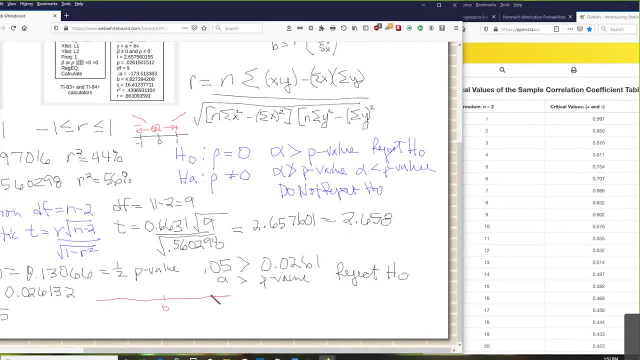 So here's 0, and they're going to give you a range. This is for 9, it's 0.602,, which means the other end is a minus 0.602.. So these are your critical values, And if, if our r value is between these two values, then it's not significant. 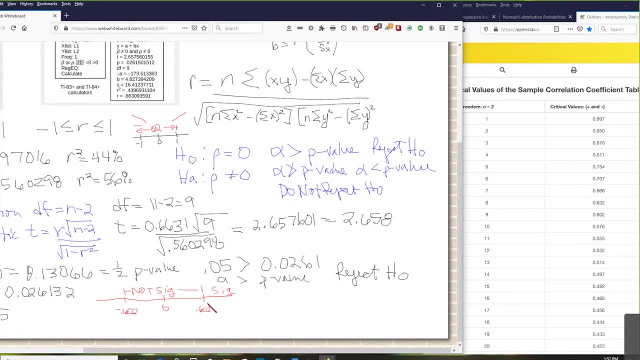 If it's outside, if it's either greater than or less than, then it's going to be considered significant. So then we want to go and look And r? r value Was 0.6631.. So that means that's going to be. we'll say about here. 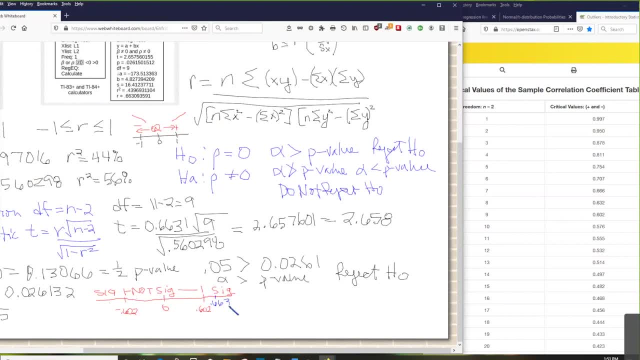 So we have: 0.6631 is our r value. So because that r value is greater than 0.062,, it's greater than then. that means that r is significant. So 0.6631. Is greater than 0.62.. 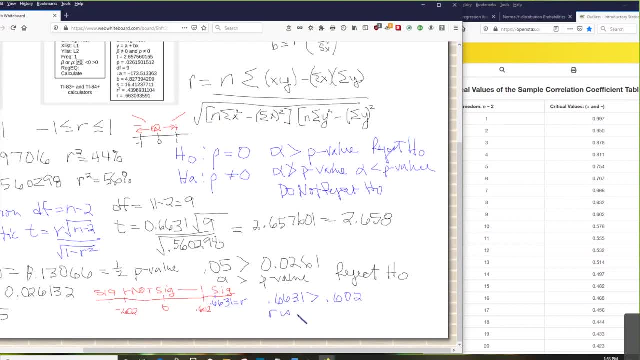 So that tells us that r is significant And that means we can reject the null hypothesis. Okay, Any questions about this. Okay, Any questions about how to use the, the table, to determine whether or not r is significant and whether or not you should reject the null hypothesis. 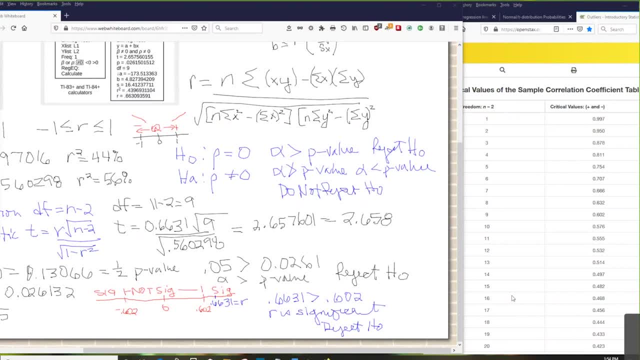 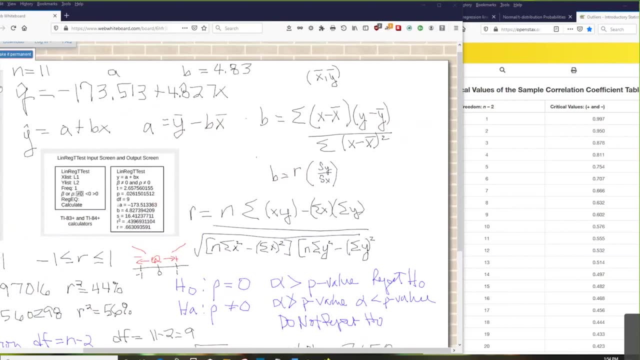 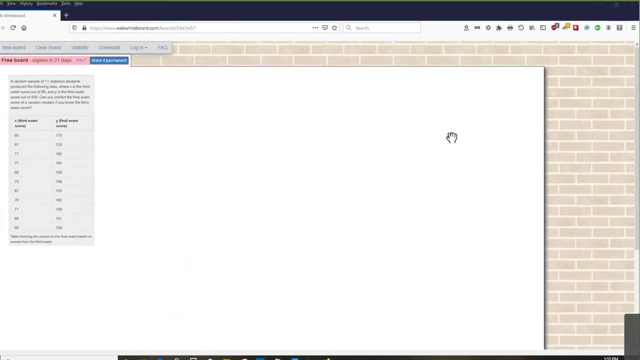 Okay, Any questions about anything we've gone over so far? Okay, So I'm going to get a new whiteboard and then we'll move on to prediction and outliers. Okay, So now we're going to look at prediction. So, because we've identified that r is significant, 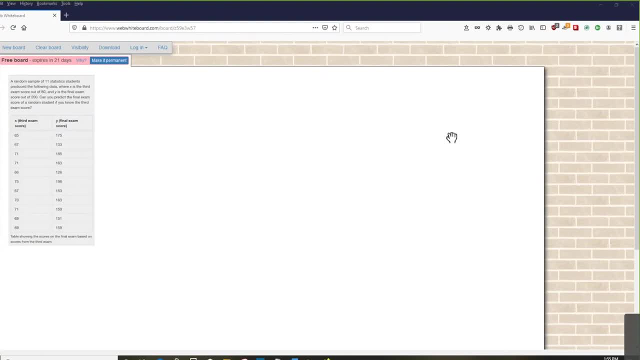 we can now use the least squares regression line for prediction. So let's go ahead and write what our equation is. Let's write that down again. So the equation that we got for our least squares, our best, our least squares regression line. 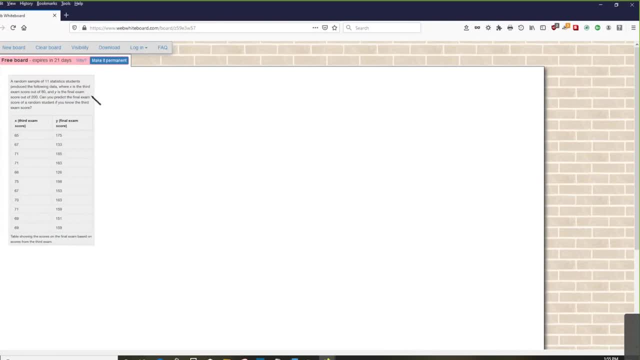 is going to be 0.6631.. So that's going to be 0.6631.. So that's going to be 0.6631.. Okay, So now we're going to look at prediction. So the regression line was the estimated y equals the minus 173.51 plus 4.83s. 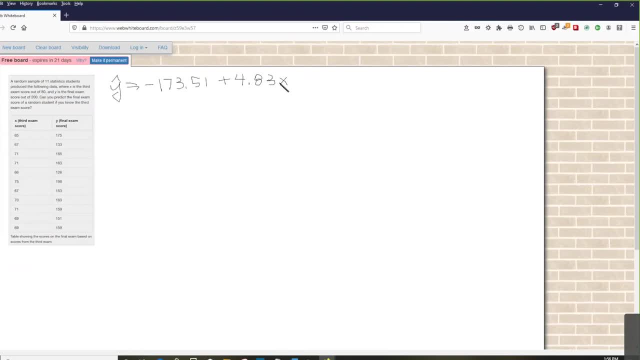 So now, when we've got so we've. so now we want to use it for prediction. We've proved that We've got everything. that's so now that tells us we can use this line for prediction. So suppose we wanted to estimate or predict the mean final exam score of the students. 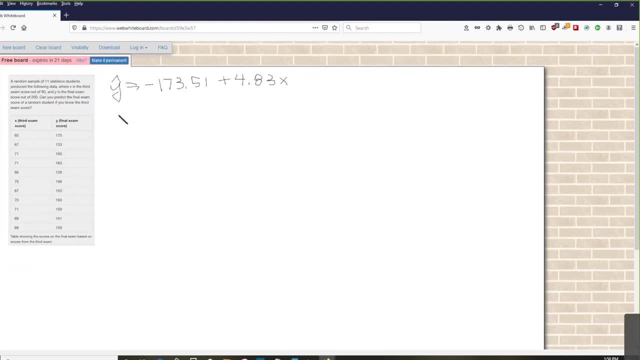 who received a 73 on the third exam. So that would be: let's say, somebody got a 73 on the third exam. Now, because our values range between 6.5 and 7.5, we're going to use this line for prediction. 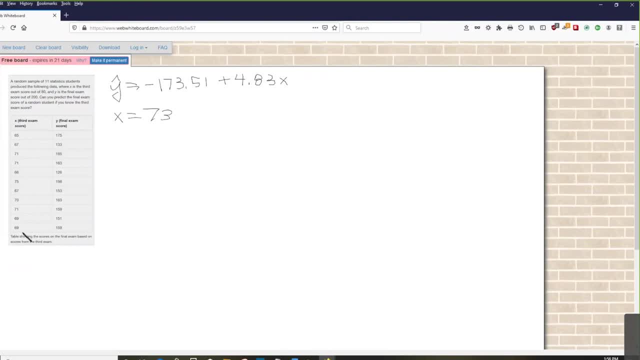 So now that tells us we can use this line for prediction. If I get 65 and 75, then that tells us that we can, that we can substitute in X, for we can substitute in the value of X equaling 73 and solve for Y to get our final expected score. 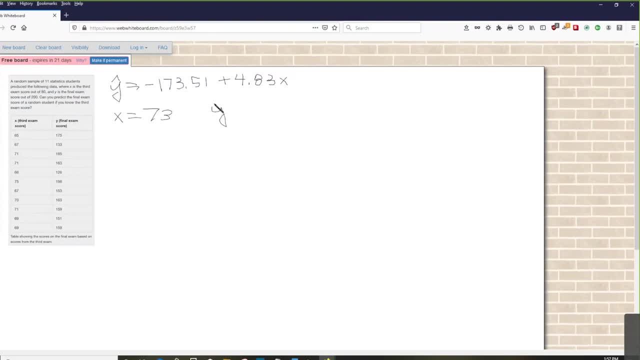 So then all I'm going to do is I'm going to take my and plug in instead of X, I'm going to plug in that 73, and that's going to give me a value of 179. oh, eight thanks. so what that would tell me is that we 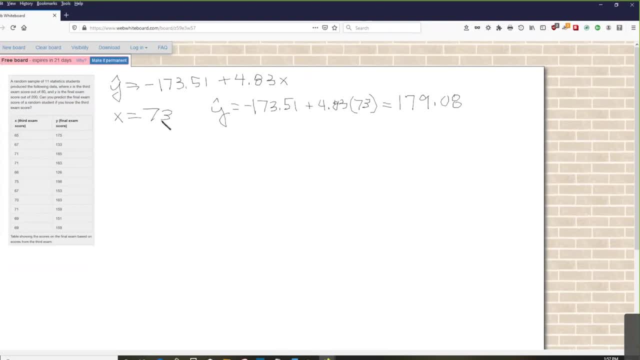 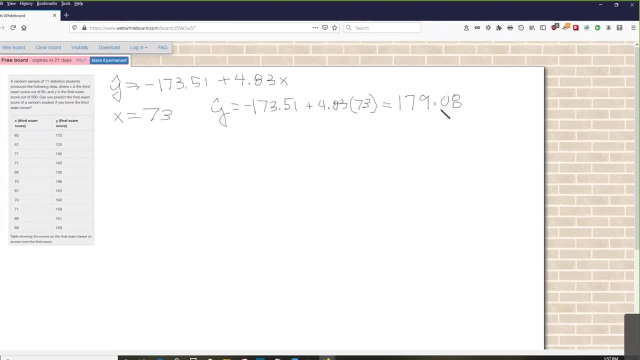 final exam. and the process of predicting inside the observed data of X values is called interpolation. the process of predicting outside of the observed X values is called extrapolation. so on this, so on. when we were dealing with our x-values, we were dealing with, we were dealing with scores between 65 to 75, so that means that anything in between any x values 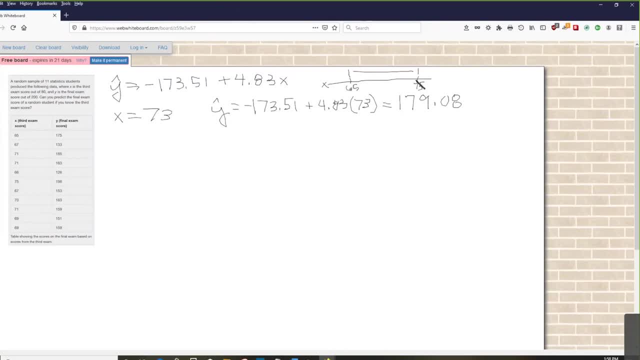 that are between 65 and 75. so in this case we were looking at 73. then we can have um, we can reliably say that, we can reliably predict what the final score is for any of these values, for any value of x between 65 and 75. now let's say: 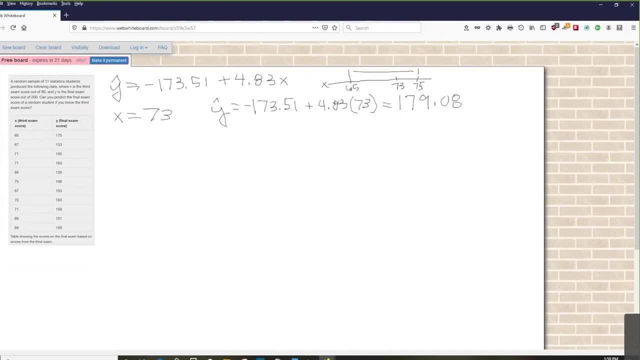 that i want to predict something that's outside of this range of data values. so let's say, i wanted to find a score that was between 65 and 75 and i wanted to find a score that was between 65 and 75, out for a student that had a score of 90. 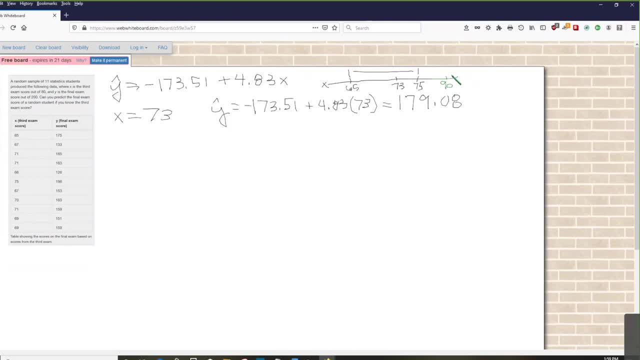 what is the likelihood? um, what is likely to be their final score? so this one, we're going to do the same thing. so let's say x equals 90, then we're going to do the same thing, plug that in and that's going to give me a score of 261.19. 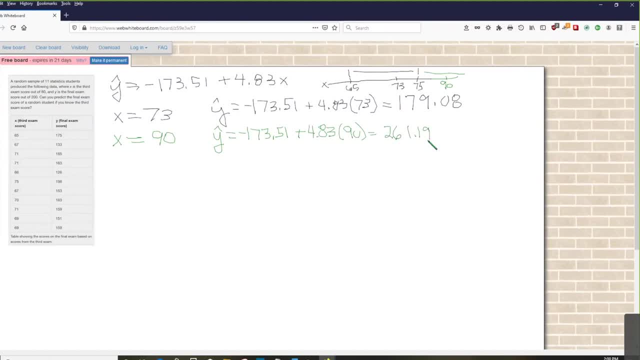 so, so we're able to plug it into the formula. however, the largest final score possible is 200, so what that tells us is anything that's outside of the range of our sample. the outside of the sample domain cannot be used to predict reliable outcomes. 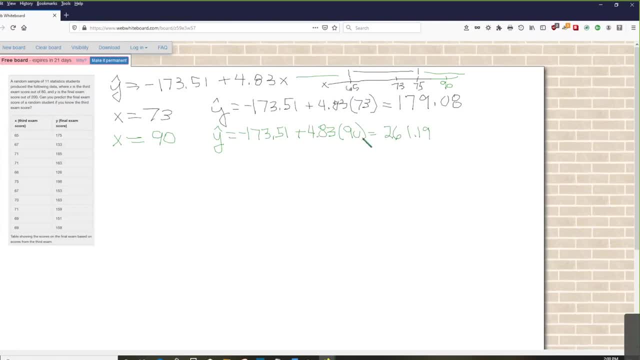 So we can still plug them into the formula, but, as you can see, all this is going to tell us is that they'll probably score high, but we can't predict what type of score that student is actually going to get, because it's outside of the range. 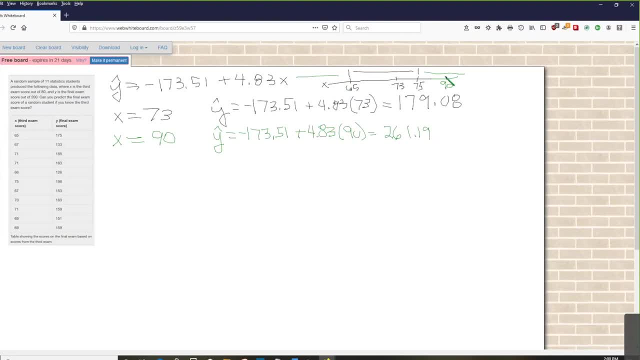 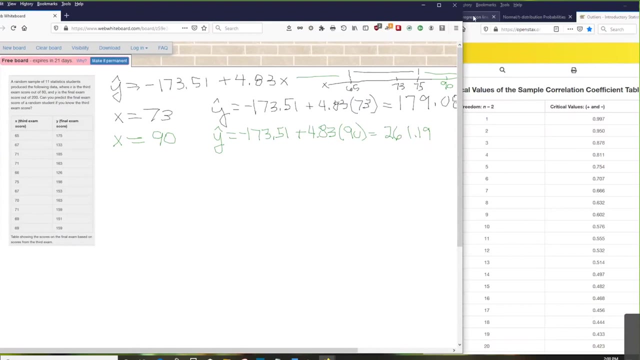 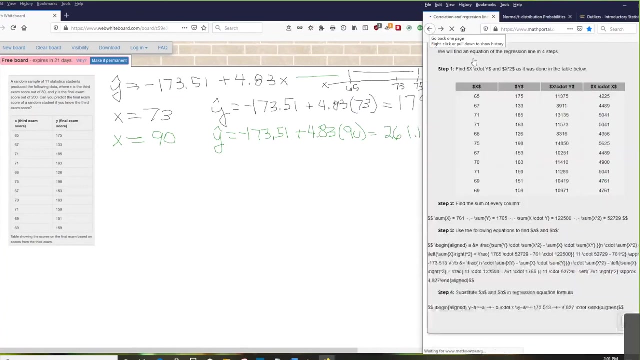 that we actually measured. Okay, The last section that we're going to look at is the outliers, And the outliers are when we have our data. Well, let's see if we've got, if it will show us the graph again. There we go. 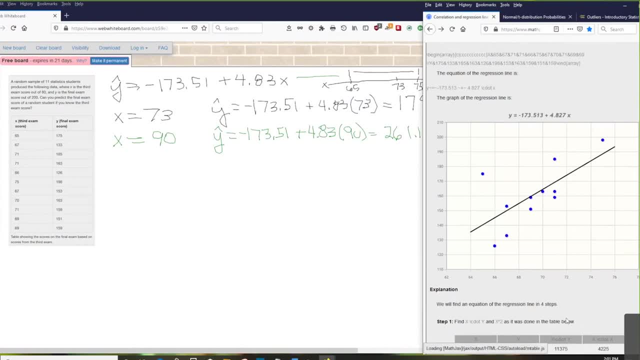 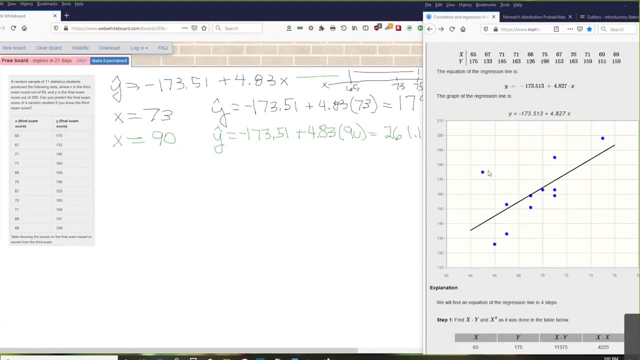 So here we have the graph. So the outliers: When we're looking at this, outliers are just the ones that are considered further away from the line And if we have an outlier, an outlier can be because we've got an error in the data. 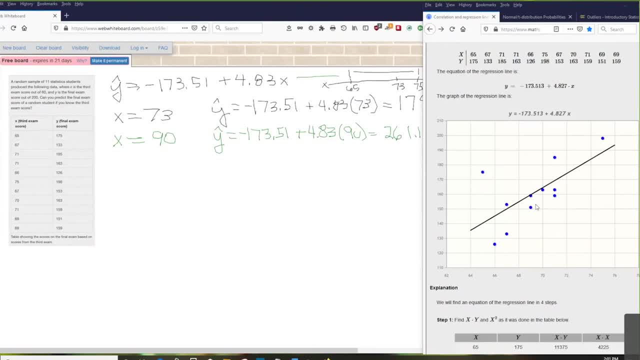 and that is throwing all of our information off, And or it could be something that's really, that's something that's important and it's influencing and having a big effect on, you know, the slope of the line. So any time we have an outlier, then that just means that's the point. 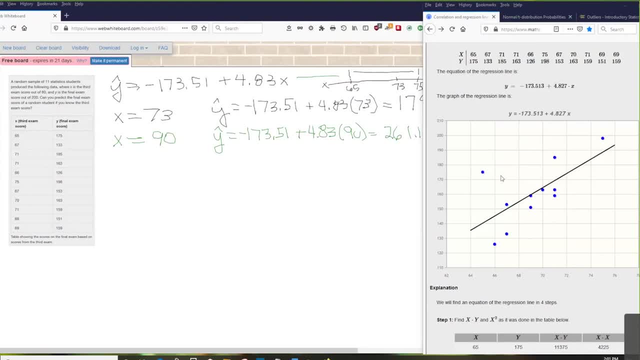 that we need to go and look at it, double check that data. So any point that is considered two plus or minus two standard deviations from the line is considered an outlier. So we can do that graphically. So let's say we have this: 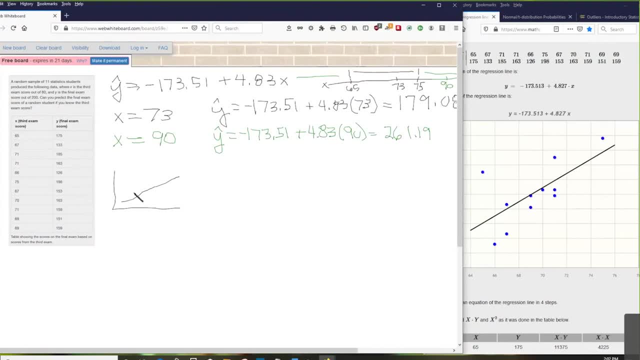 So we've got our main line and we have all our points. So graphically we could do it: make a parallel line above and below- That's two standard deviations- And then just look at anything that's above or below those lines would be considered outlier. 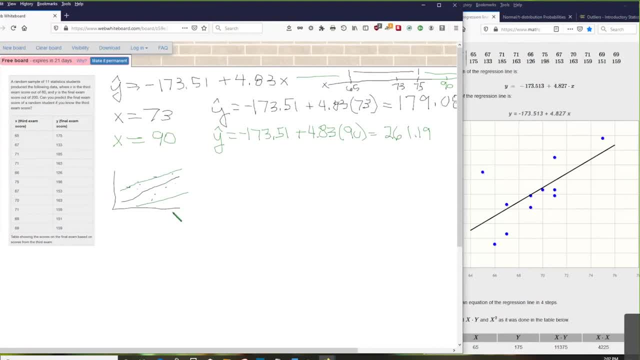 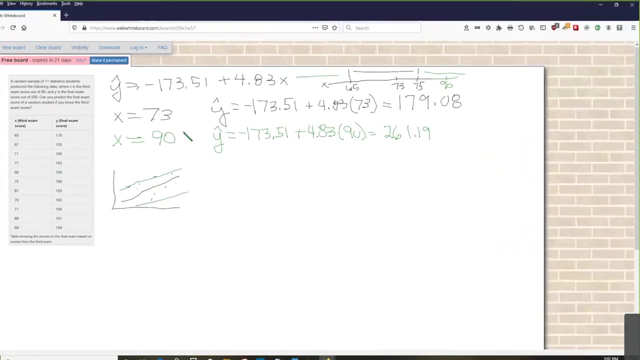 Okay, So We're going to use this sample again and the standard deviation. so, if we have, if you use the calculator, it's going to calculate the standard deviation for you. So let me pull that up again and show you where that is. 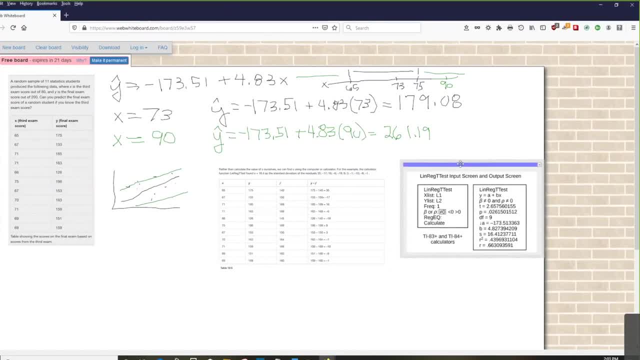 Okay, So if you Are using the calculator, then this S value where it says 16.41237711, that is your sample standard deviation. If you don't, if you're not using that calculator, then you can do it by hand. 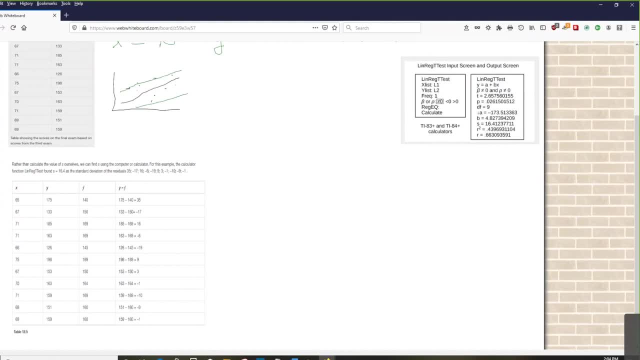 Okay, So S is the sample standard deviation of all of the epsilons, or all of the summation of the y minus y estimate. So it's what it's doing, is it's summing all of the differences between the points. 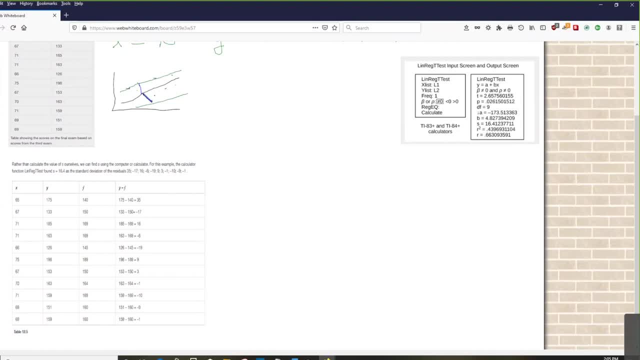 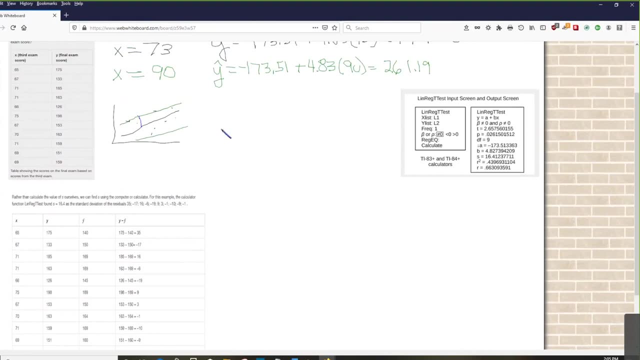 the data point and the straight line. So n is going to be our total data point, And let's go ahead and write down some equations. So we've got: n is our total data point. Okay, So we've got: n is our total data point. 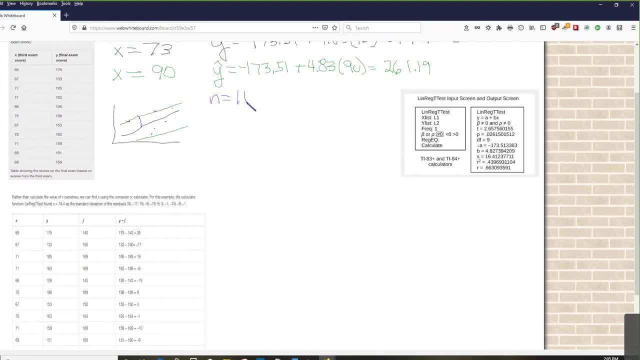 Okay, So we've got n is our total data point. So we've got n is our total data point. So we've got 11.. And then our formula for our sample, for the sum of the squared errors is going to be the sum. 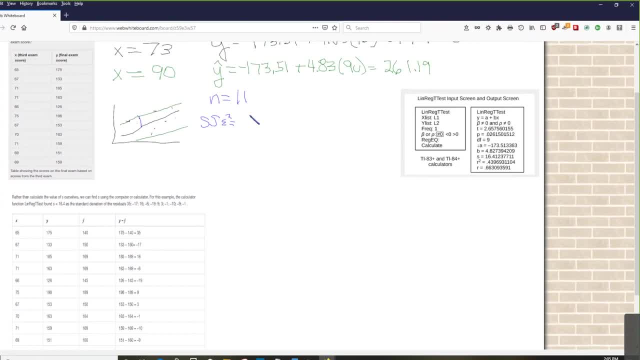 of our epsilon squared, which is just the summation of the squared differences, And then the formula for our standard deviation is going to be the square root of our sum of the sample errors divided by n minus 2.. And once again we're doing n minus 2.. 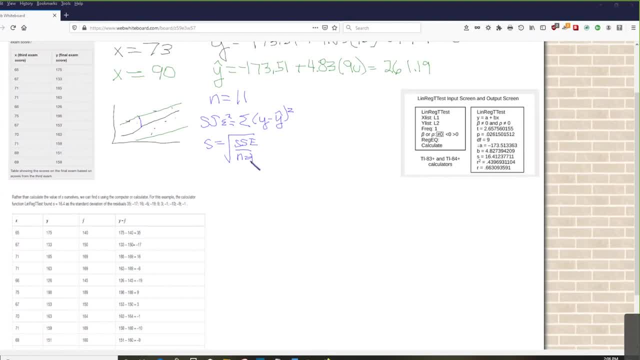 And then, if you'll remember so, this is the same as doing the square root of the summation of the data point minus the y from the line minus the line squared. So this is the distance, or the error, between the data point and the line squared divided. 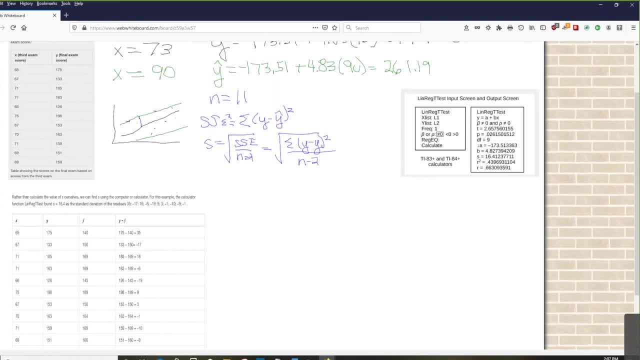 by n minus 2.. And then, if you'll recall from module 2, just to see how this looks familiar- the sample standard deviation for module 2, when we did it, that was just the value of x minus the mean of x, quantity squared divided by n minus 1.. 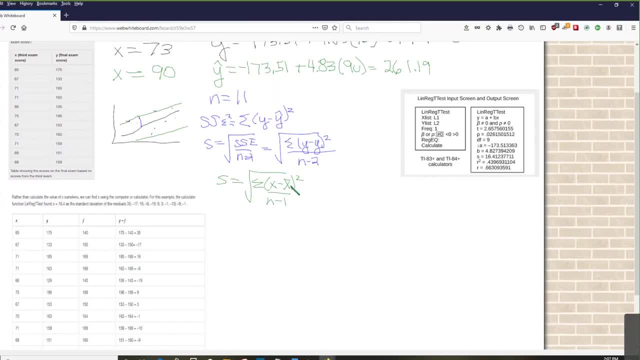 So if you're working just with one value instead of two values, you're going to use this equation for your sample standard deviation. If you're using two values, you're going to use this top one in blue. OK, So now. so from this one, the calculator gave us a sample standard deviation. 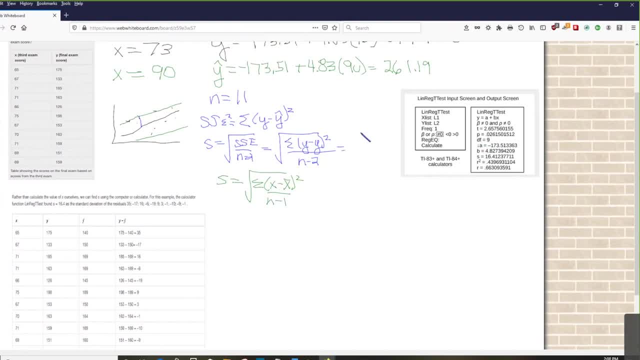 Let's do it in the same color of about 16.4.. So now, if you don't have that calculator, then you will need to do it by hand. So let's go ahead and do that. So this table did a bunch of the math already for us. 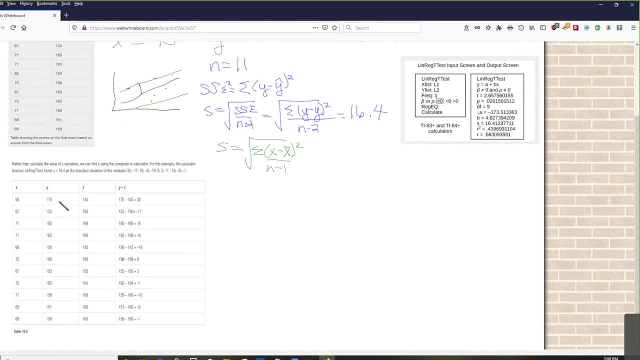 So this is showing these are our x values, These are the y values. This is the estimated doing our equation of the line. It plugs that in for y And then it took the differences of those two y's and gave us the differences. 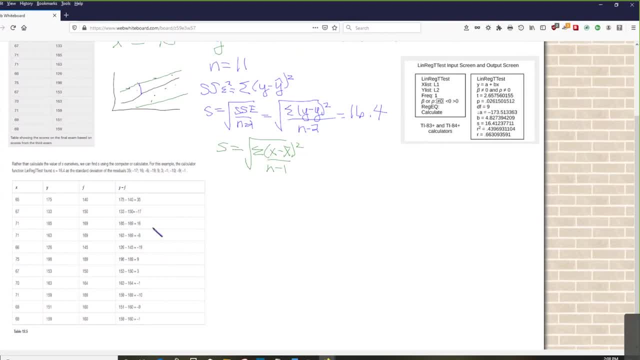 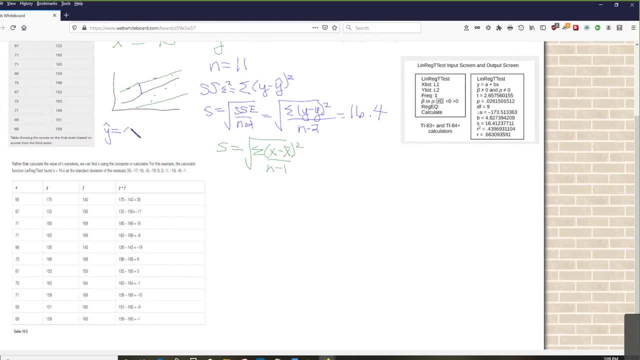 So now let's go ahead and do that. So my equation is just your a plus bx. that we solved earlier, So now we've got the epsilon. So in order to get my sum of the squared errors, then I'm going to take each of these values, each of these differences. 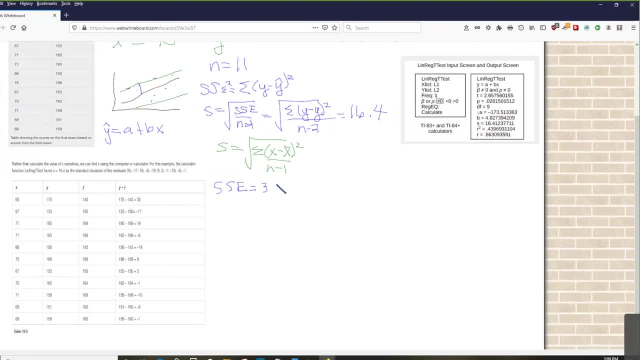 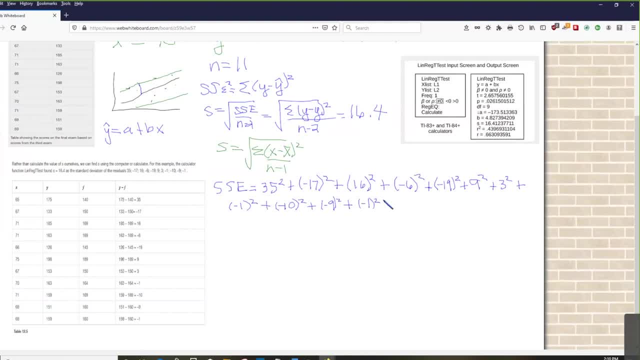 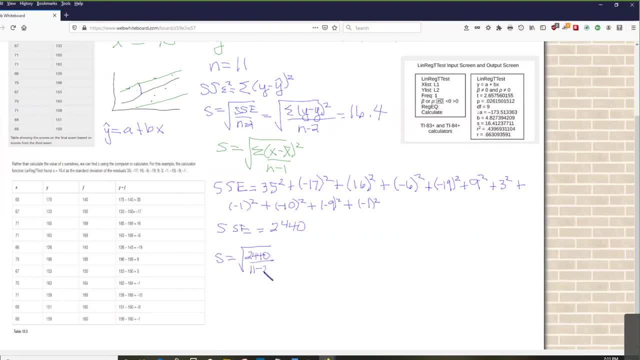 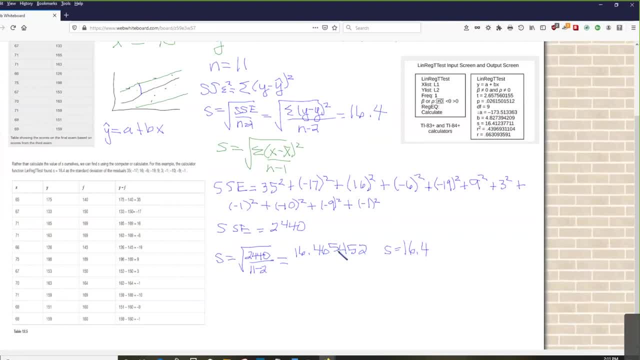 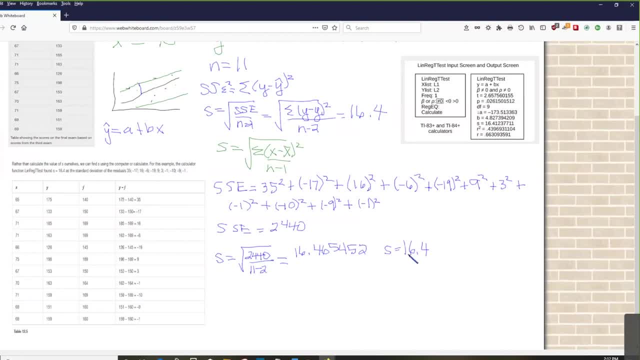 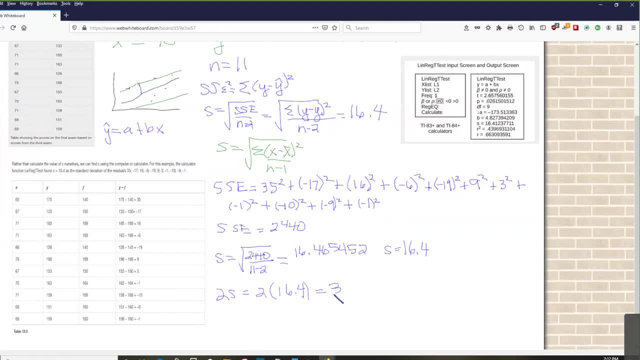 score which equals 32.8.. So now I'm looking for any score that is going to be plus or minus 32.8.. So now we look at all of these scores and we can see this first one is bigger than 32.8,. 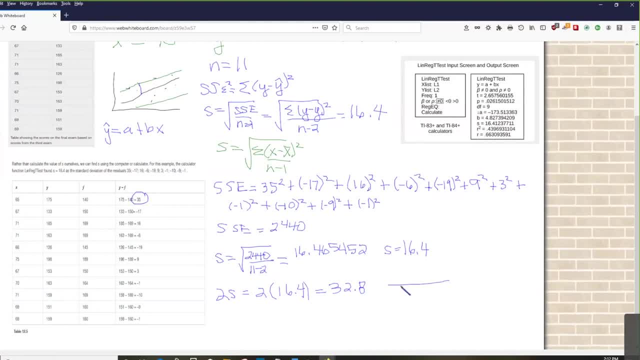 but everything else that we're going to look here. So this is zero. so we want minus 32.8 and plus 32.8.. And we've got a value of 35 on this first exam. So that tells us that the first student has a residual of 35.. 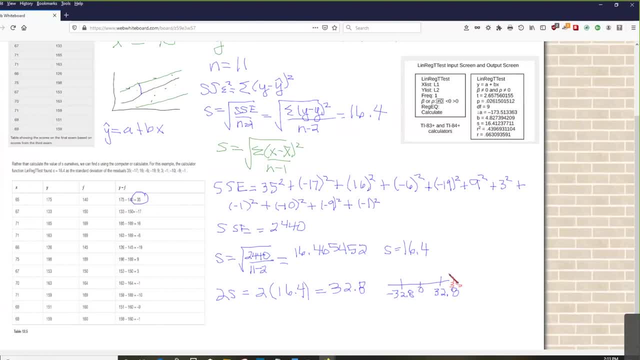 And residual is just the term for the difference between 32 and 32.. The data point and the line it's referred as epsilon. It's also referred as a residual, So that would be considered. so that tells us this point right here. 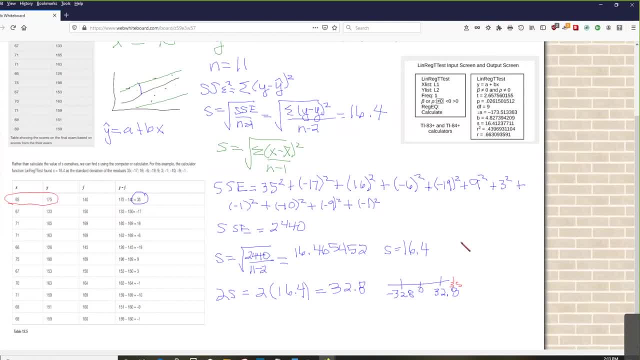 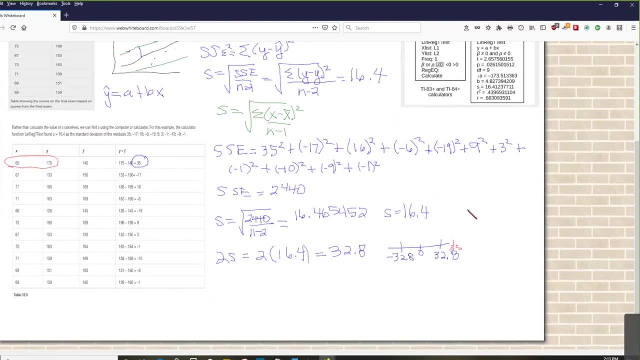 So that tells us that. that tells us that point. So that's what we're going to look at. Let's look at this graph. So we have the value now at sixty-five. Sixty-five, which is our x value, and 175 is considered an outlier. 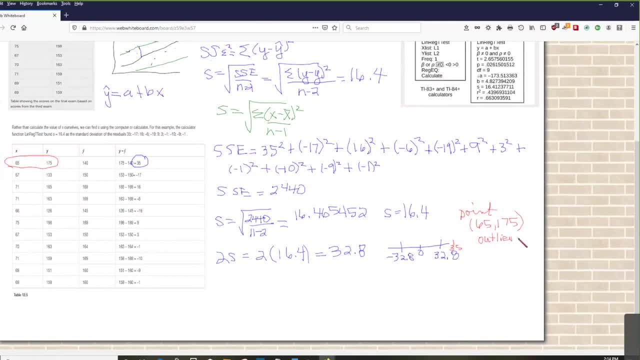 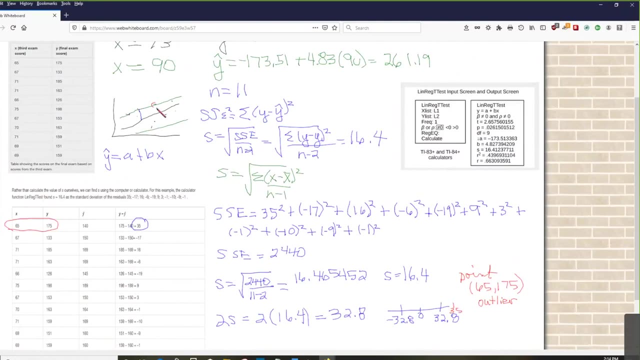 Because it is more than two standard deviations. it is more than two standard deviations away from the line And sometimes you can visually see it on a graph, but sometimes like say this point right here where it's physically there. We'll try to get the average values to be on this graph. 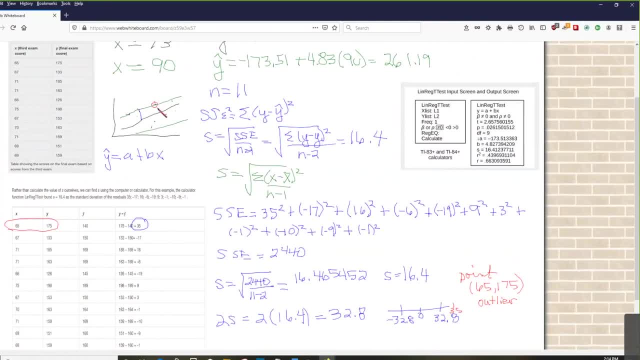 just barely above that line. that might be kind of hard to visually see it, but your calculations will identify it. So if you have an outlier, then that just tells you that's the data point. you need to take a look at it. If it's an error, then either you need to correct the error. 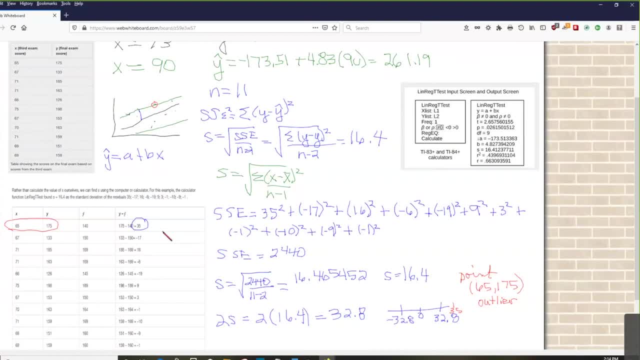 or you just need to delete it from your data and recalculate without that data point. If the outlier is not an error, then you want to make sure that you leave it in the data set and see what it tells you about how it's changing the line. 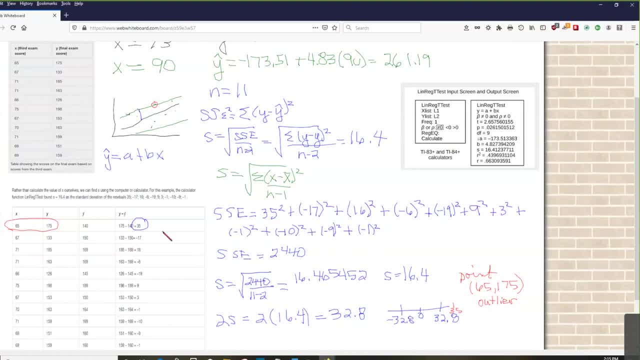 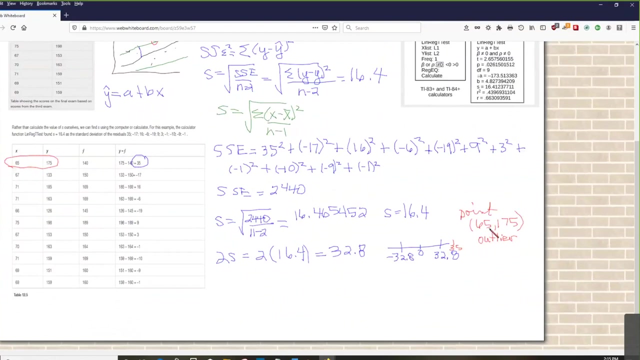 And you can also take it out and do your calculations and compare it with and without so that you can see how is that outlier affecting your best fit line or any of your other data. So just for theory, let's suppose that our point 665175 is an error. 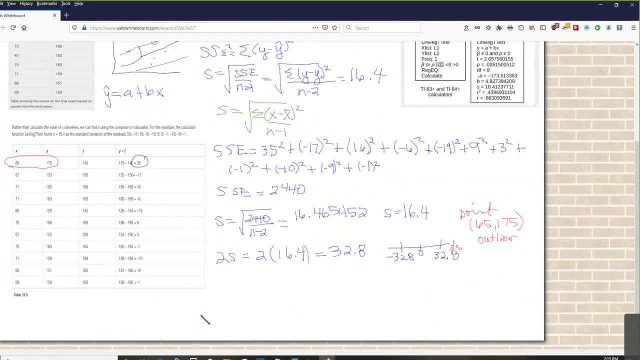 Then we're going to delete the data point and recalculate it. So if we recalculate it we'd put it back into our calculation. So let's look at what we had. So that would give me. so, without the outlier, then I would get a new line of minus 355.19 plus 7.39x. 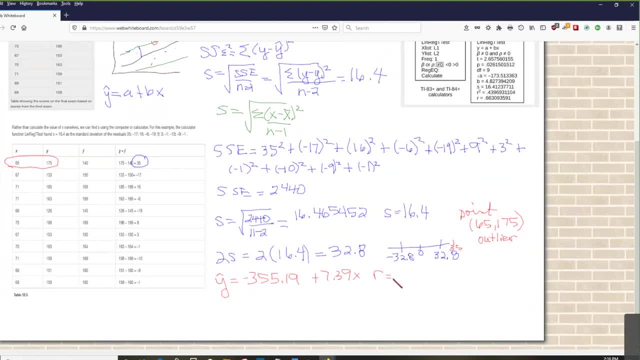 and a correlation coefficient of 0.921.. And then what we had originally. we can do it again. Finally, just so we can compare it, we had a minus 173.513 plus 4.827x, with a correlation coefficient of 0.6631.. 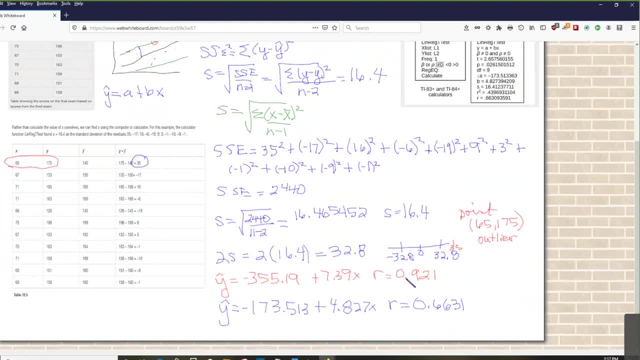 So when we compare this to data we look at by taking the outlier out, we actually got a stronger correlation coefficient because r is now much closer to 1. And this also tells us that this line will better predict the final exam scores given.